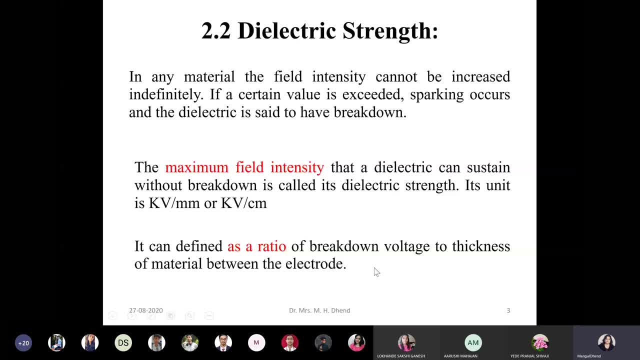 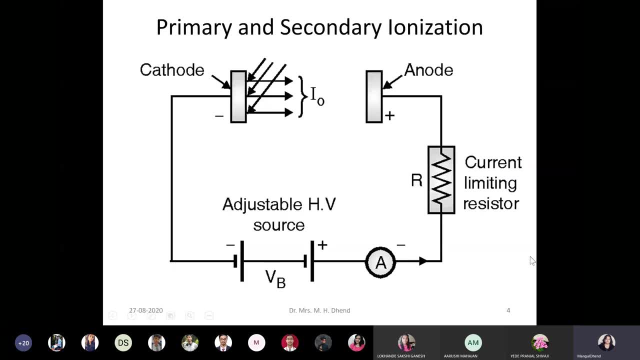 by the gap distance. So we discussed primary ionization and secondary ionization. I will just revise when you will apply very high voltage supply. If you are across the electrode, where electrode material is between the electrode material is air, then air is having 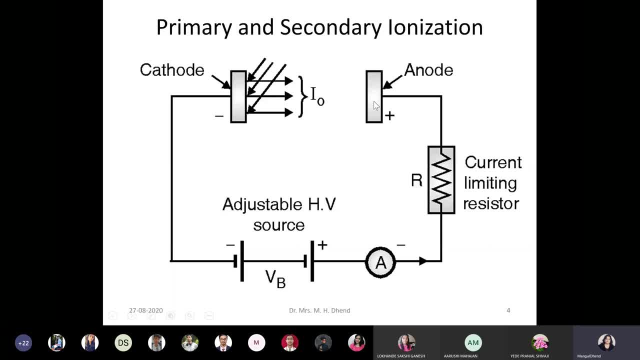 gas molecule, and gas molecule means positive central charge nucleus and surrounding is revolving electron. So how this primary ionization and secondary ionization or breakdown process start? initially you are just thinking. first step has to occur, That is, initiating electron in the gap. Who will throw initiating electron in the gap? How it will in the gap, That is. 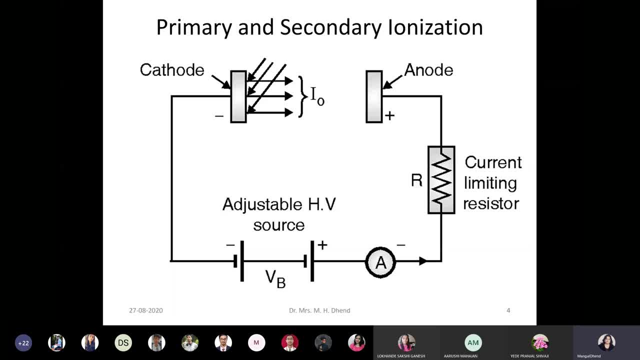 unpredicted means. it is statistical in nature And depending upon that statistics, you will get breakdown voltage. so you are exciting your electrode with illumination because when you are conducting experiment, illumination is there, light rays are there, sun rays are there. so due to that, this electrode surface is having made up of metal and metal is also having a central charge positive. 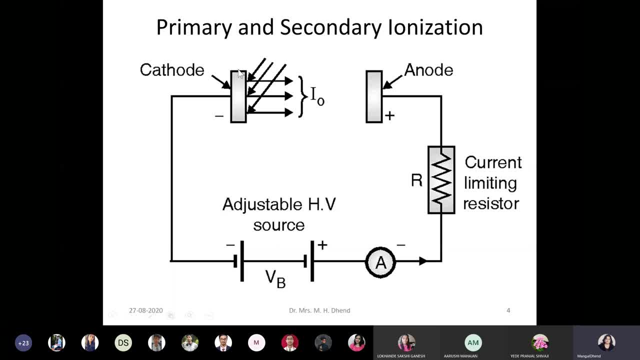 nucleus and revolving it electron. but when revolving electron gets energy from the light radiation, that electron will get excite and then it will become free, because here positive charge is there, so force of attraction to the revolving electron of this electrode surface is there, and when you are applying very high voltage, this voltage is also very high and then it will be. 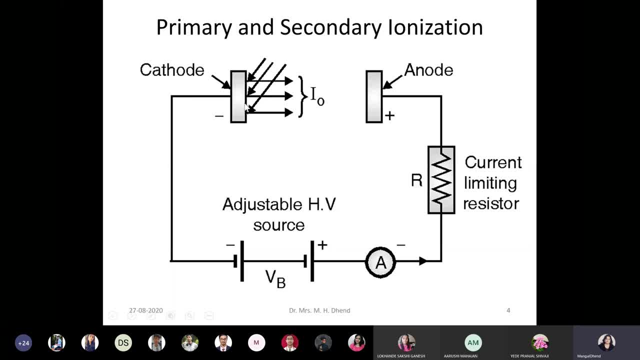 successful to drag the electron from the cathode surface and that electron will be shifted, drifted, attracted towards anode. So therefore one initiating electron will be there. then, while traveling towards anode, it will collide with the gas molecule. again, it will collide with the electrons revolving from the gas molecule. 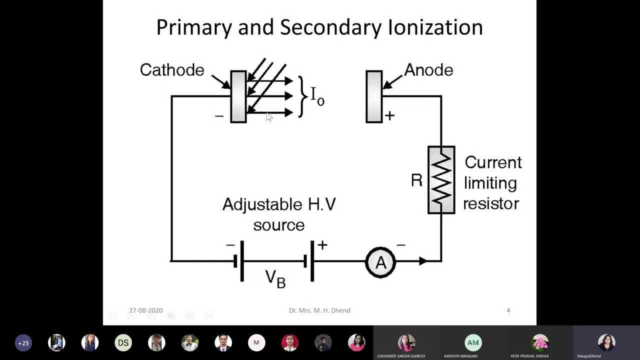 and it will disload the electrons from the gas molecule because when it is running towards anode it is having kinetic energy. that kinetic energy will be given to the electrons from the gas molecule. So level of energy of the revolving electron from the gas molecule will jump from valence band to the conduction band and again electron from gas. 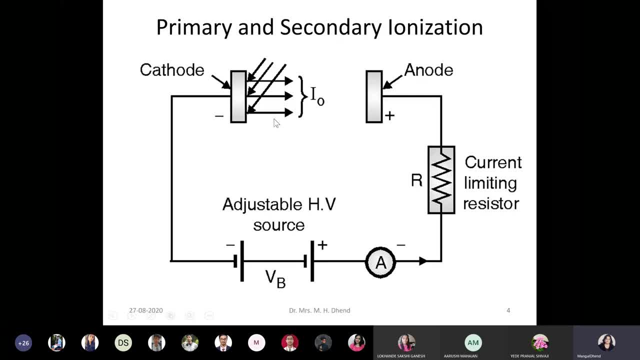 molecule will rush towards the anode. So when electron crossovers the gap, by that time positive ions central from the gas molecule will be there in the gap, but they will also get attracted towards negative charge cathode. So electron will rush towards anode and positive ions will rush towards 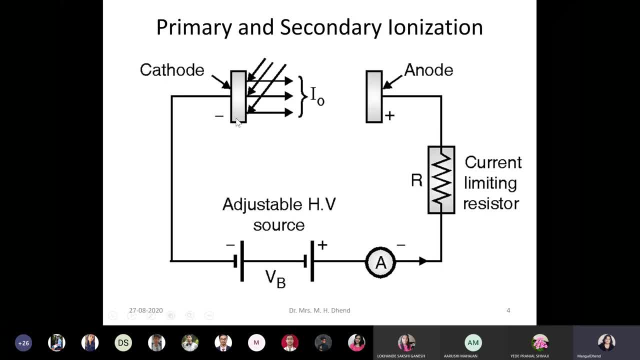 cathode. So there are two process: primary and secondary ionization. When initiating electron collides with gas molecule and electrons liberated from gas molecule, that is primary ionization. and when positive ions bombard on the cathode surface and it will liberates electron from cathode surface, that is secondary ionization. So that we have discussed and breakdown will take. 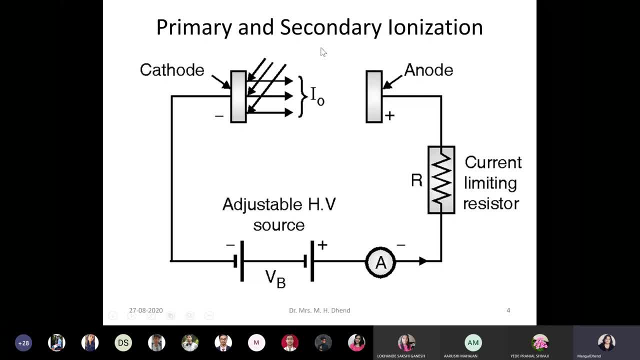 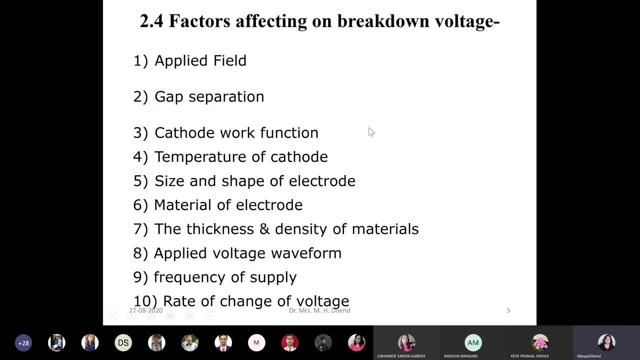 place Factors affecting on breakdown. we have discussed applied field gap separation, cathode work function, temperature of cathode, Size, shape of electrode, material of electrode, thickness and density of materials, because if you are testing air, you will get different voltage. If you are testing liquid, you are 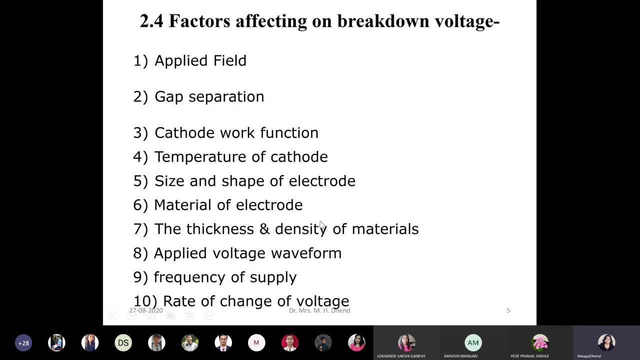 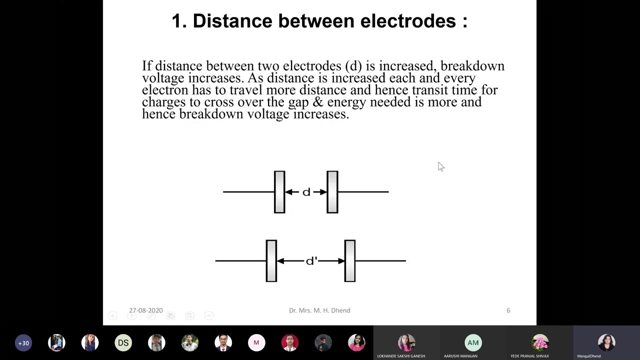 getting different voltage Applied. voltage waveform is also important. Frequency is also important. Rate of change of voltage is also important. So read this. So we have discussed factors in detail. If distance is large, then breakdown voltage will be large, Because electron has to cross over from cathode to anode. So here, if you will see one, electron will 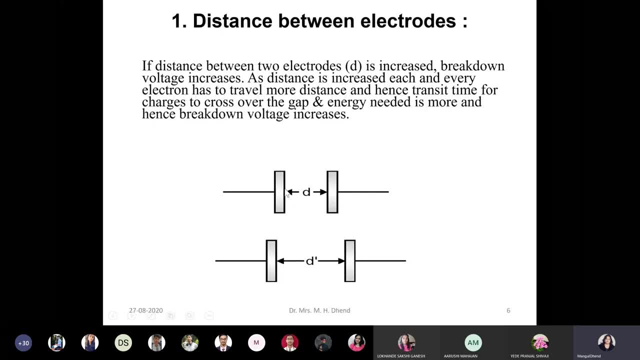 reach towards the anode immediately. but if gap distance is more that electron has to cross over larger distance. So definitely large voltage has to be here across this. So breakdown voltage you will get large if gap distance is increased. Then shape of electrode we discussed If diameter of 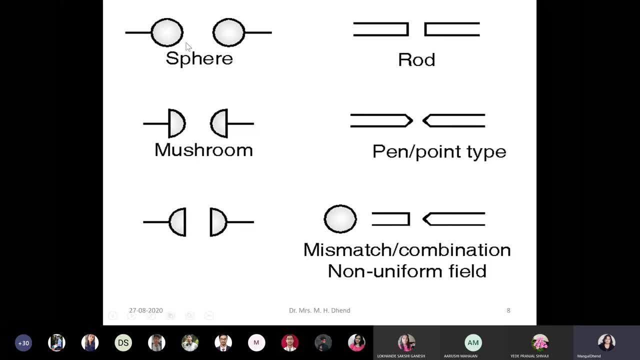 electrode is more. you cannot say that gap distance Will change. When we discuss effect of diameter, you have to say gap distance remains same, Other parameter will remain same, Material will remain same. Simply, you are increasing diameter and gap distance is same. Then what will be effect? So if you will see diameter is increased, then you can. 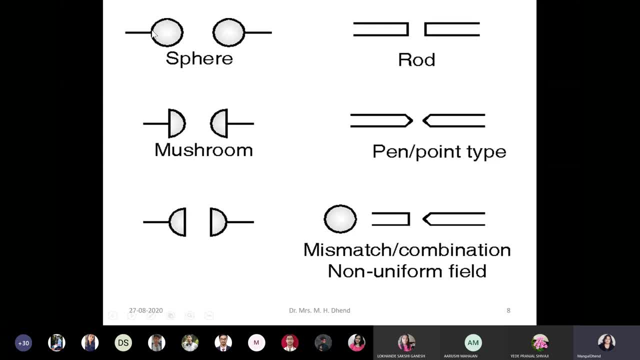 see this, perpendicular distance will change. So you can say: as perpendicular distance is increased, number of gas molecules will increase. and due to number of gas molecules are increased, now more electrons will be available And breakdown voltage will be less. But reverse effect is also there If diameter is increased. 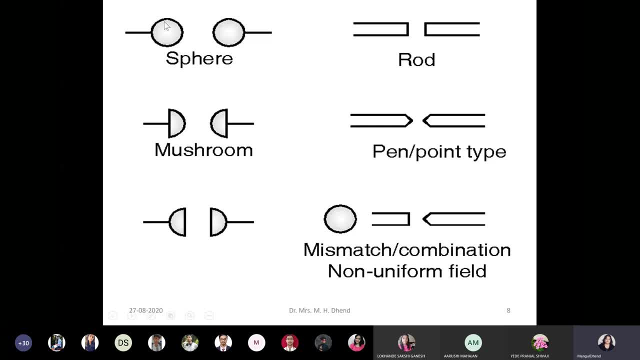 intensity across this electrode will be reduced, Because intensity means this perpendicular distance. you will consider What will be voltage divided by this perpendicular distance. And if diameter is increased, this perpendicular distance is reduced. So E will be higher If perpendicular distance is increased, if diameter is increased And intensity will reduce, And as intensity 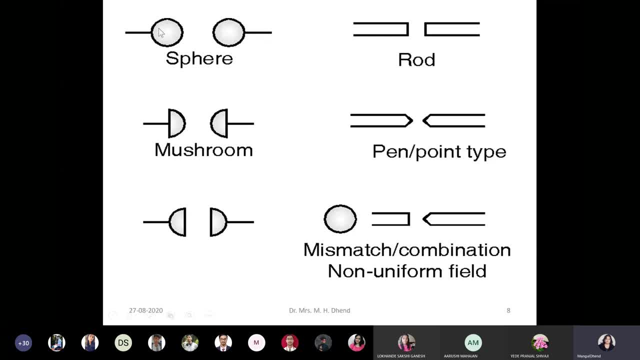 will reduce, you will get breakdown voltage will increase, Because less intensity means less force. Dragging force will be less. So that way you can see here, If radius of curvature is small, intensity at this tip will be very high, And we have discussed in this case breakdown voltage will. 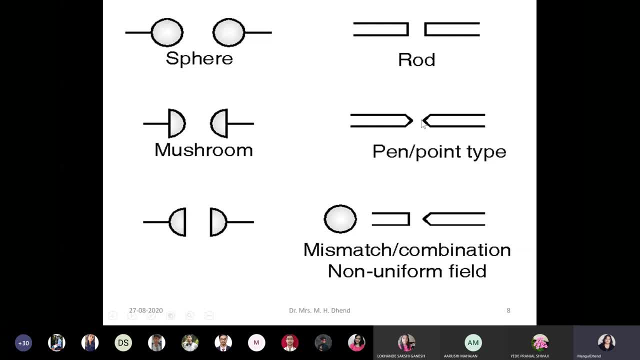 be very rapid, Because even if you are applying 30 kilo volt, intensity at this will be very high as compared to this electrode. So breakdown will be here, 3 kilo volt, and here you will get 30 kilo volt. So now again it is possible to reduce this voltage, But you have to pay attention to one. 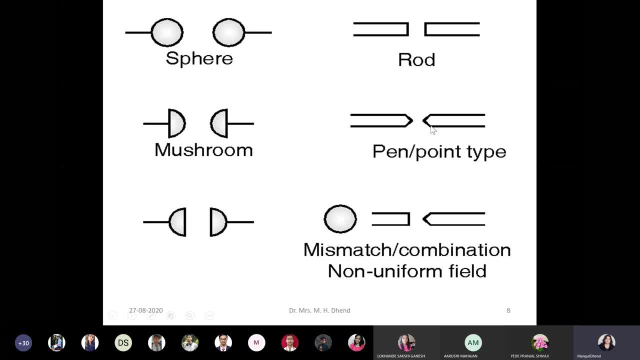 thing, It is very important that you will not apply pressure every time, Because all the holes are made of a same material, Same gap distance, Same other things, pressure temperature up here. So non uniform peel is not desired in our applications Because it will reduce the dielectric strength of. 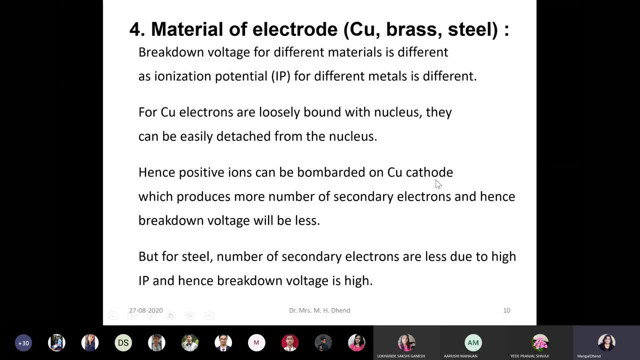 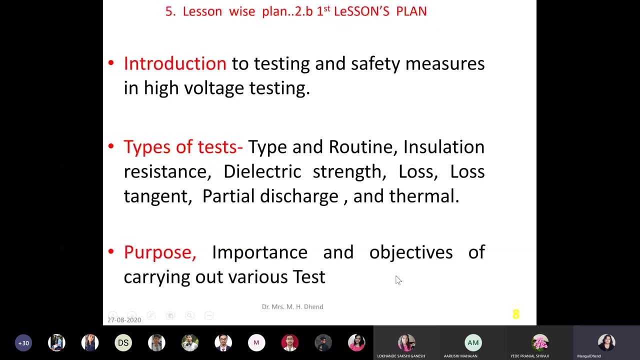 the material, Then size of electrode. just now I discussed Material, also discussed- Read this. so i discussed what methodology i will use: memorization catch-up video we played. we have also seen competition. we also saw who are the active persons and how retic immediately jumped. 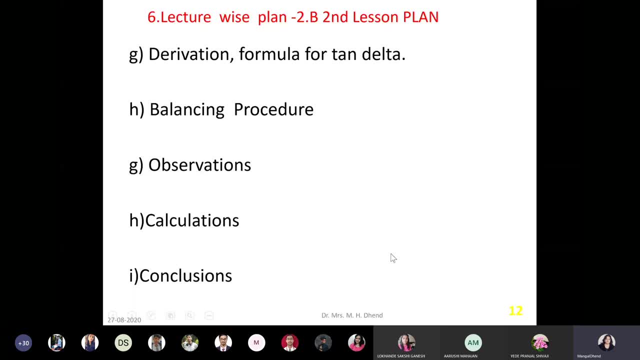 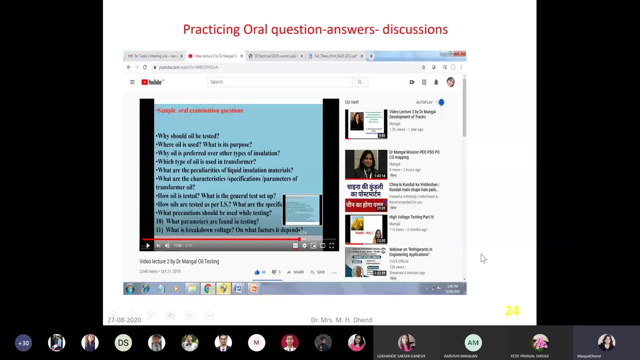 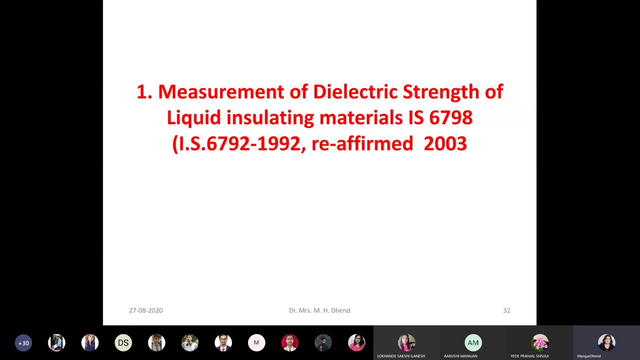 to the first level. that also we have seen. so let us see today what happens. so all these things i have discussed, books, i have told you now refer the is. i am giving you a hint: remember is for liquid which is used. you have to remember this year and number. okay, this is six, seven, nine, eight. 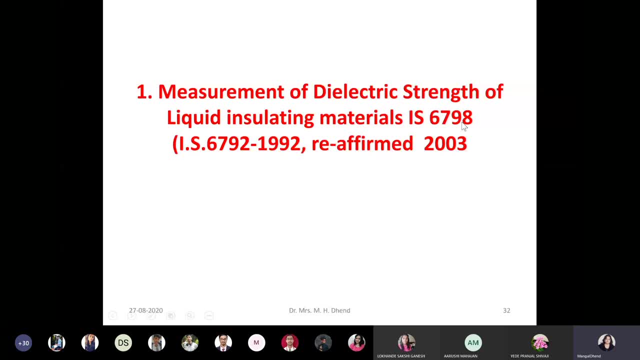 but it is reaffirm. in 2003 means, if you remember this number, year is this otherwise, earlier was this number and in 92. but you have to remember, remember devices. so we have discussed breakdown voltage, how to find out of oil and as per is method. also. 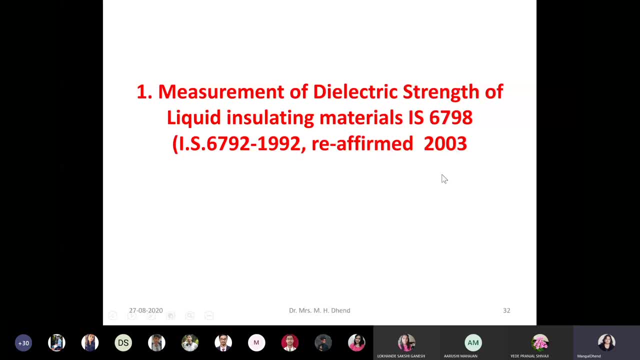 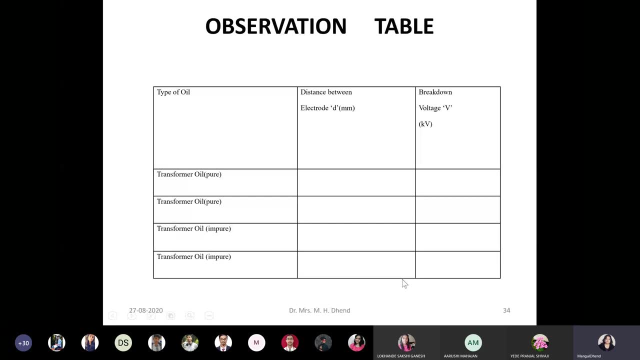 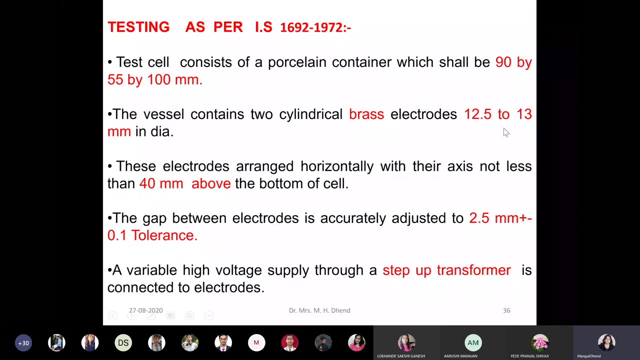 we have discussed: what is the distance of electrode, what is the diameter of test cell, what is the electrode material shape diameter, what should be the gap distance and what is should be? the tolerance means positive. negative tolerance means this: 0.1 higher or less, you can. 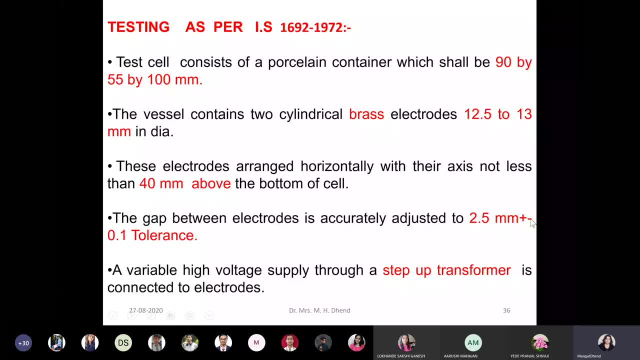 not accept level of oil 40 mm above below step of transformer, then the rate of change of voltage is 2 kilo volt per second, because if you will vary with another rate, breakdown voltage will change. meter gives rms value, so that we have already discussed it. and if you will test for oil testing, 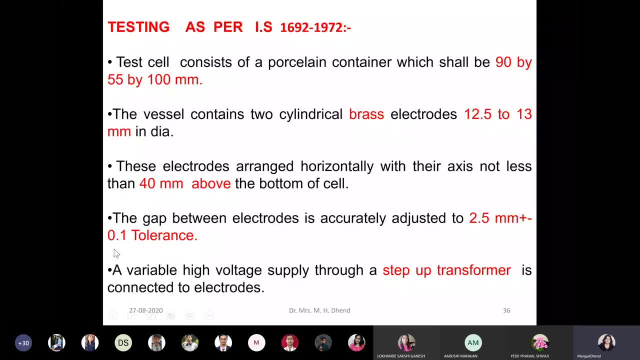 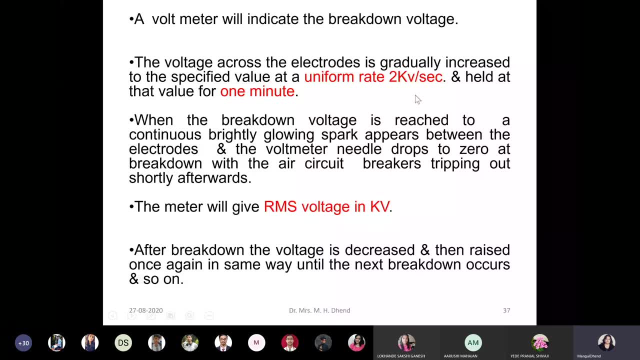 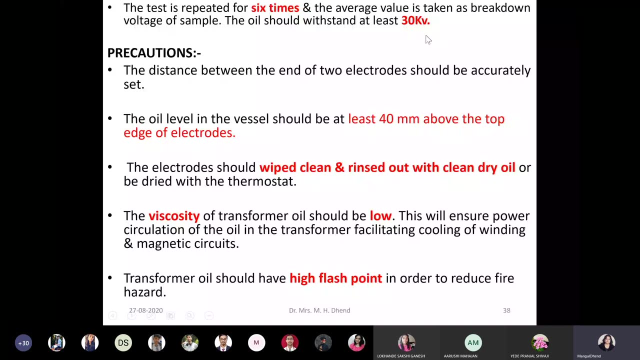 six times readings are required and if you will test as per is, then your oil should withstand the kilo volt. see generally. actually, for oil you can remember 40 kilo volt and air, you remember 30 kilo volt. okay, so while you remember 40 kilo volt and air, you remember 30 kilo volt. 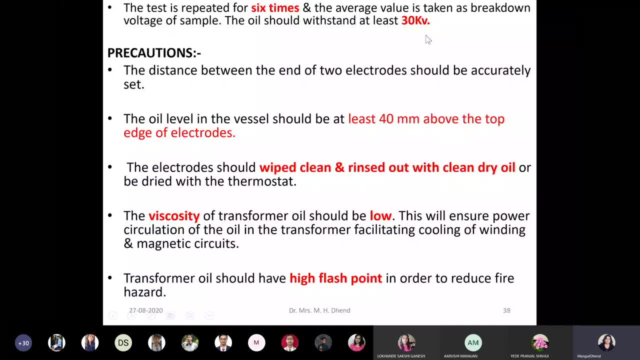 so these oral questions and videos are there. on oral discussions, videos are there now. you played a competition also today. i have added a few questions in that, so we'll just see that then. solid material testing is: is this: you remember and be honest yourself. don't refer, don't copy. 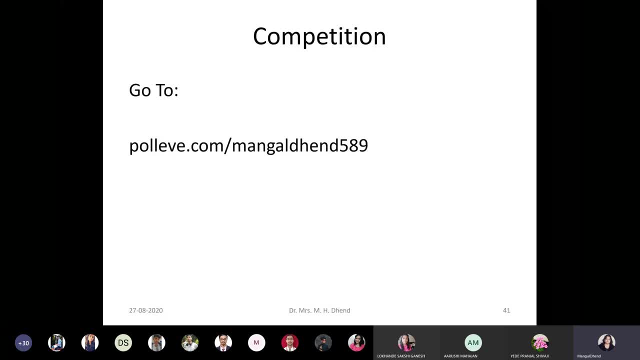 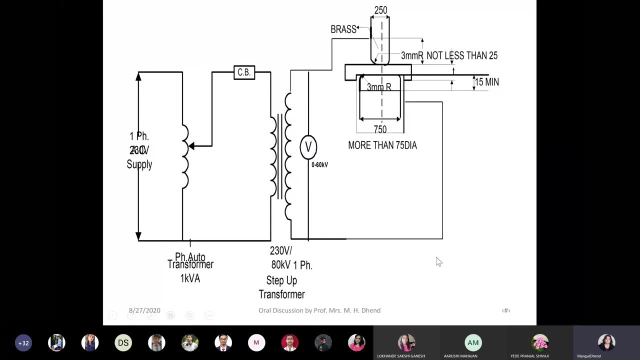 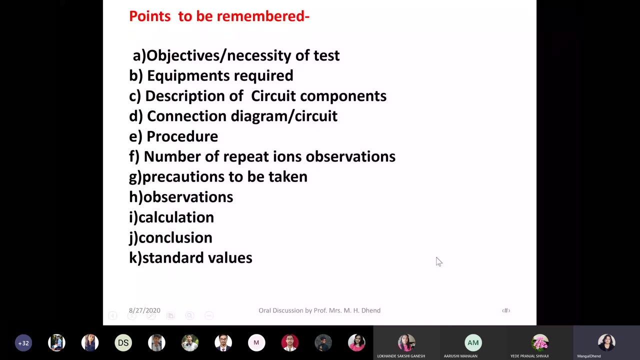 for the test. if you will just go on doing that, that is not going to help you. because what is important here? your brain exercises are important. why i am wasting so much time asking you question and just making you recall, because these are brain exercise. if you will just go on exercising daily, then your memory 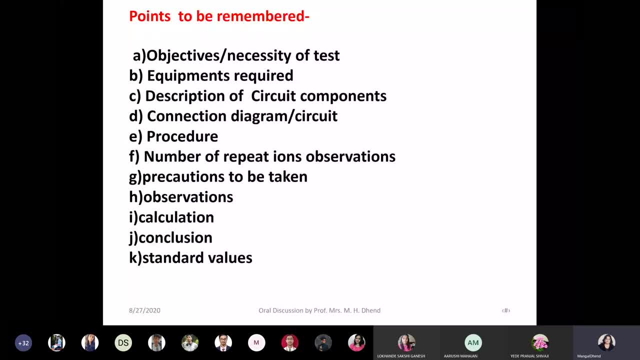 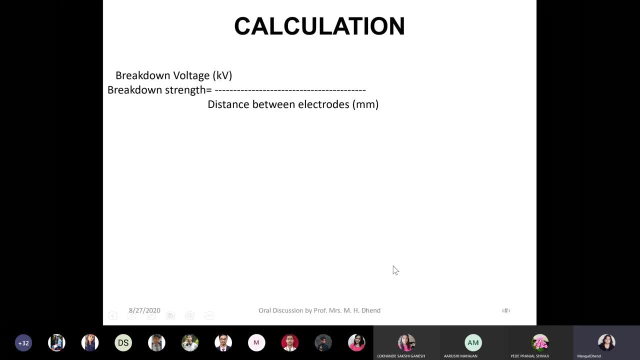 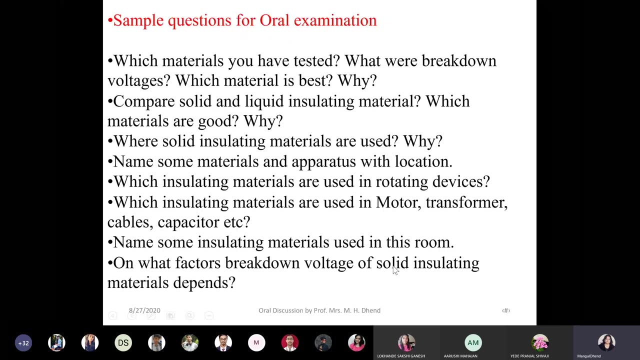 will shut and it also helps you to remember the data. but if now you have kept notes in front of you or some snapshots, and if you'll give test, neither brain exercise will be there and neither you will remember there what should be our ultimate aim. our ultimate aim should be good. 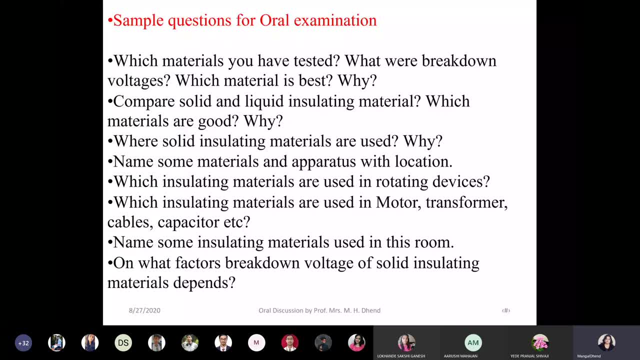 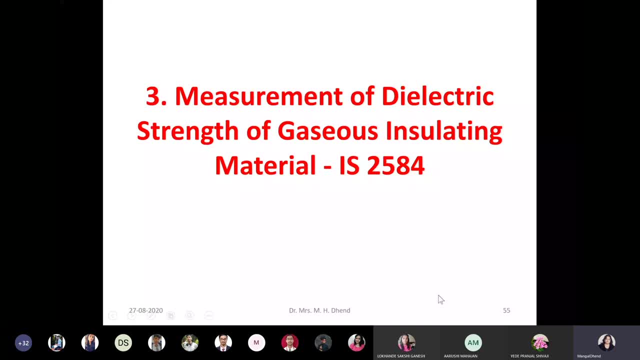 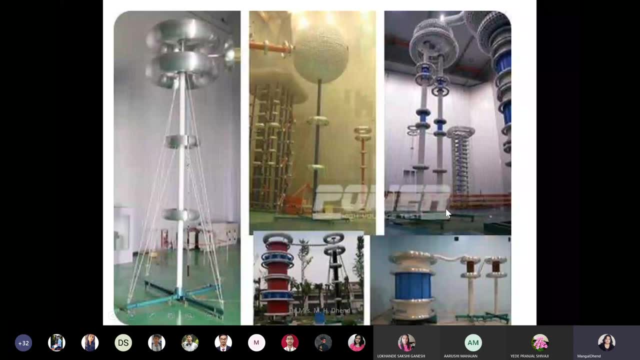 success. good memory power. that should be ultimate objective. don't keep your aims very low if you'll keep one minute paper also. i took and in one minute paper i got very good feedback. but i also got some suggestions. not should be uploaded. actually i had uploaded for force unit. 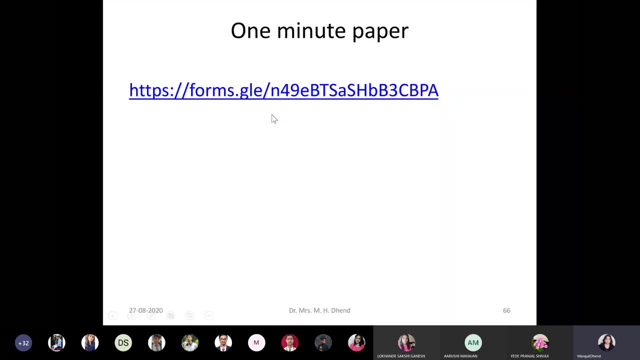 late because my objective purpose unit was different: to generate a point generation skills and also memory maps and also assignment was there self-work i was expecting, so i just uploaded late. but for a second unit i have uploaded write-ups. have also uploaded. go through the google classroom. 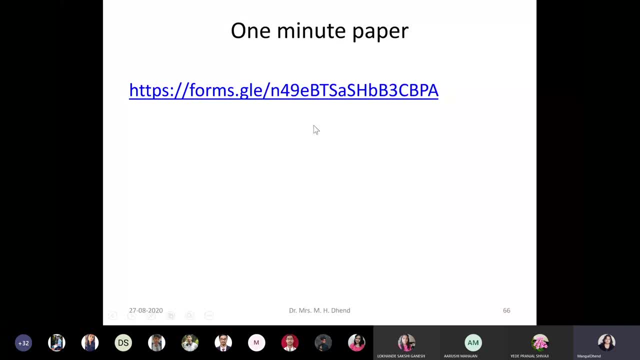 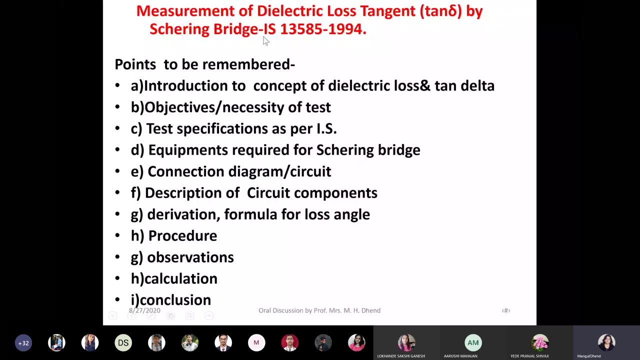 in detail rubrics and future plans also i have uploaded. so go through the classroom uploading google classroom. then sharing bridge: we discuss, remember this size for sharing bridge, and then i explain this: Electronic Laws: we were asked to think about this and just i explain this: del Hendrick clause: see, remember formula: tan delta is equal to iron. i see, i have given. 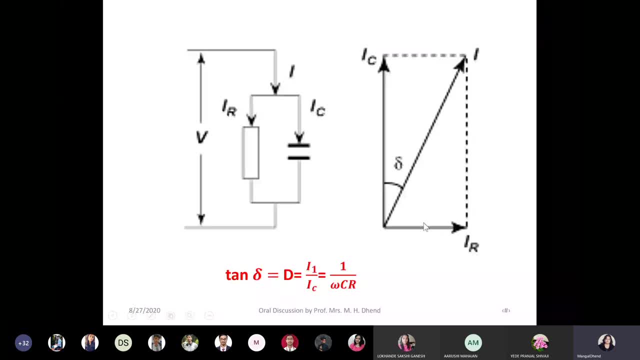 little homework for you, because that again will start from the first unit and i am going to check that your homework in first unit because again we have to discuss this little so loss tangent tan's- influential, we have seen it measure with How to remember the formula I told you. 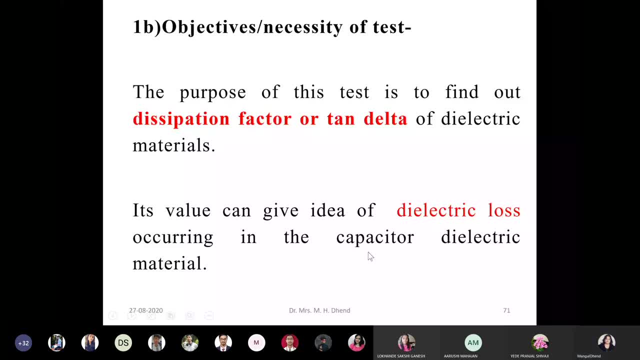 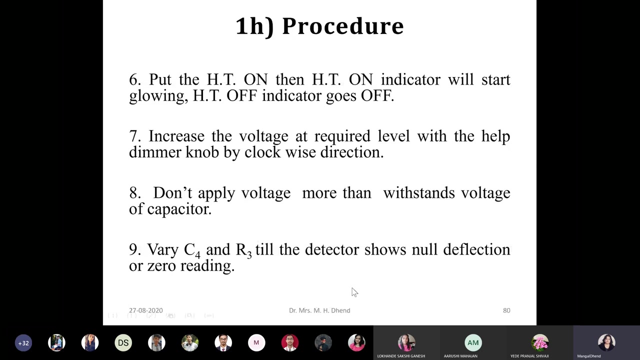 What happened? Hello, Can you see my slide? Okay, I'm using my backup network and backup network is weak. My primary network is not available today. So, procedure: we discussed Then this. Okay, now just watch the video, or some actually. 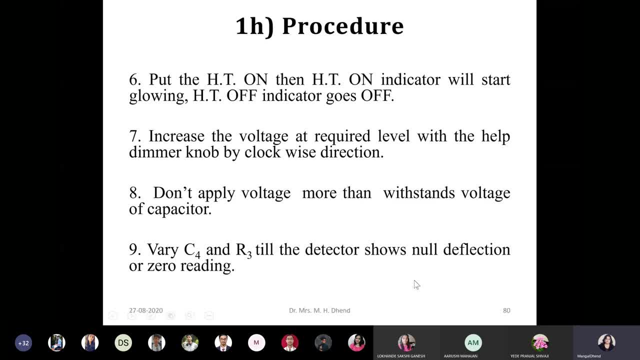 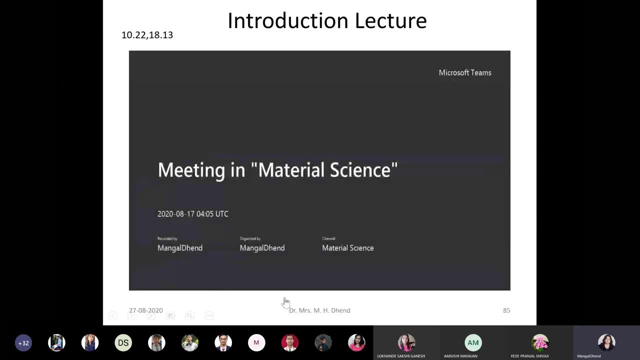 mentally wanted me to tell you this- that she is at her native place, So there is no network there, So she couldn't give the test today. She tried to log in into teams as well, So she just went to a Google class and ended up reading it as well as Google Classroom. 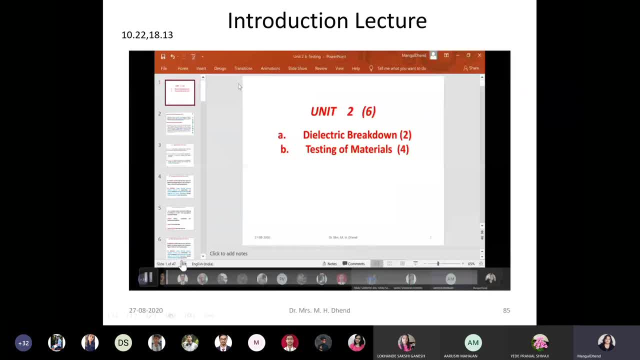 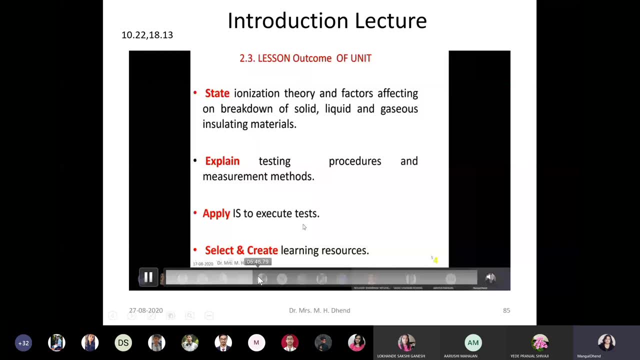 standard. So again, now that that is approaching 20th, I was you complete and say it is completed. You have created very good learning resources. It's because you will get mark, Declare our foot and then point generation Get you no point. We'll take job, Don't just log in. 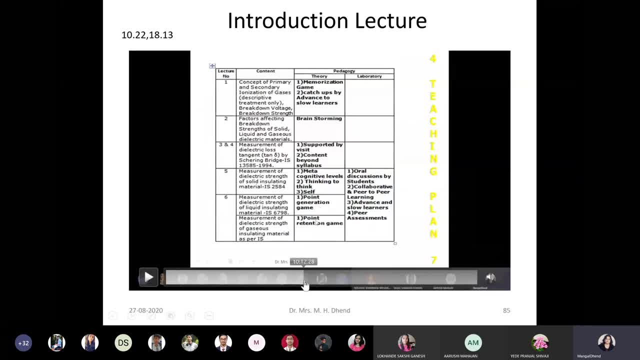 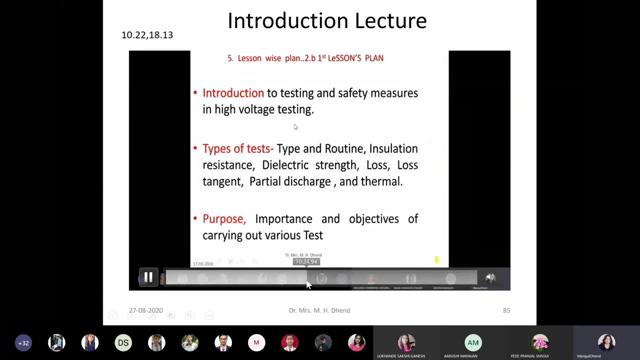 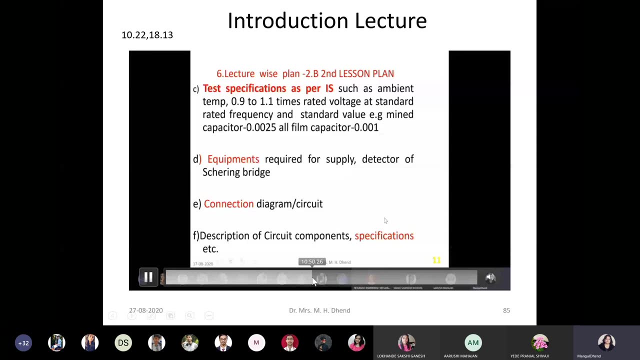 I will come to know now who has only login And then listen my plan I have made. Now listen my plan for You should able to write down the test with equipments, which equipments we use, what should be connection, how to draw circuit diagram. what are the specifications of each device? derivation of formula: if required, what formula? that is only for 10 delta. 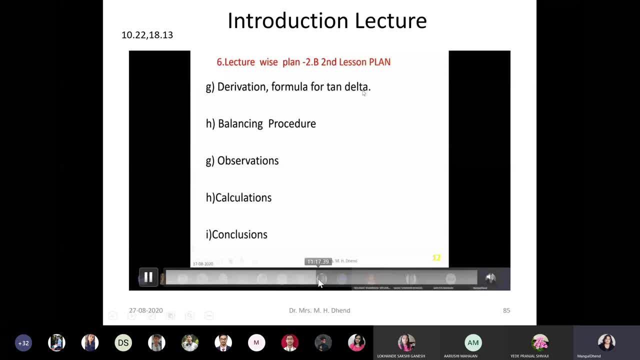 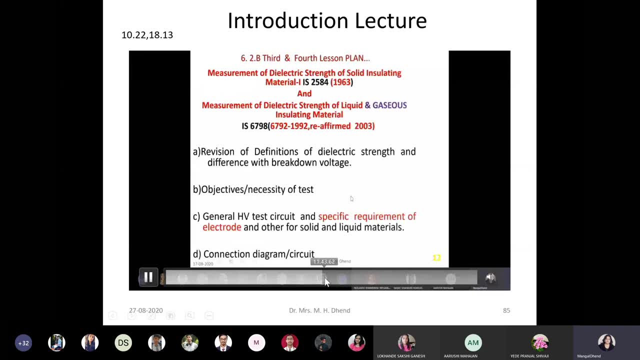 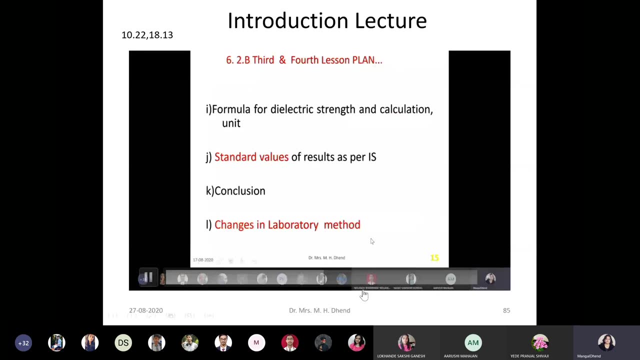 Then balancing procedure. if procedure we have to follow point, you must able attending lectures, what you can write down that. So that is what I wanted to tell you: my objectives now. what will be teaching activities? So just now we will start with my one video of oil testing, because I am starting with first test. 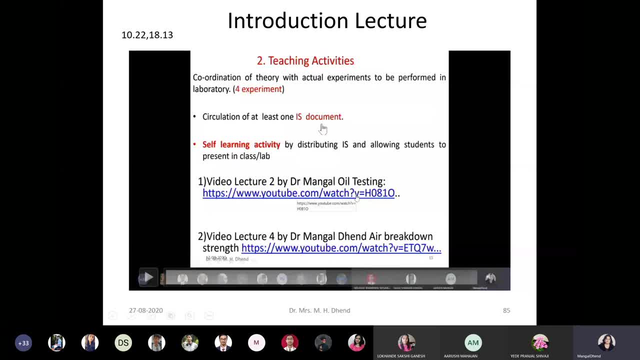 I am uploading today IS. I will just scan an app, we will upload an. You carry out one activity if you are opting it for your optional activity from our part B, So that way you can go and you can take it IS activity if you are interested. 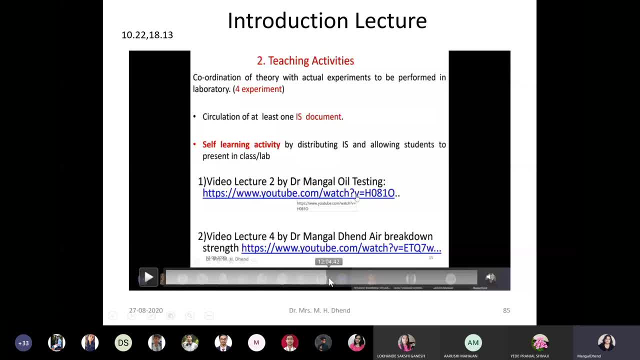 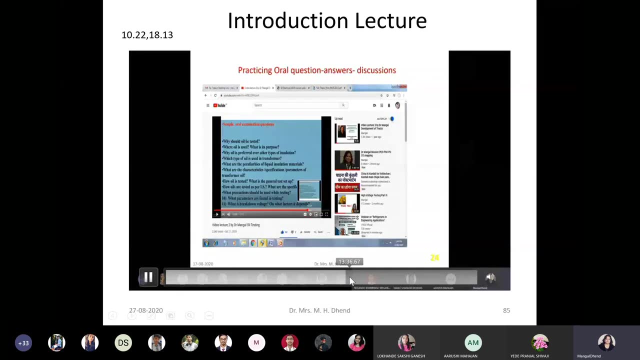 Already I told you you select your activities. Three activities you need to select, three compulsory. are there Turn voltage of oil. So first you watch the video before we start discussing that experiment. okay, Pressures equipment Proceed because second, discuss in the lecture better understanding the oral questions students expect will be there. okay, 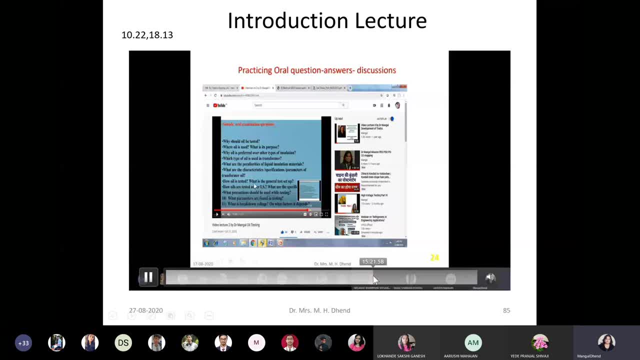 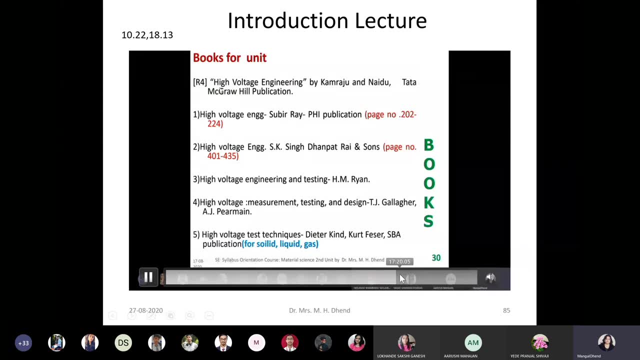 So now books For this unit. you must refer high voltage engineering by Kamrojanadu that you ask me scan copies of this book for the unit. content of Okay. now video. I have seen only Venkata and Sushmita and 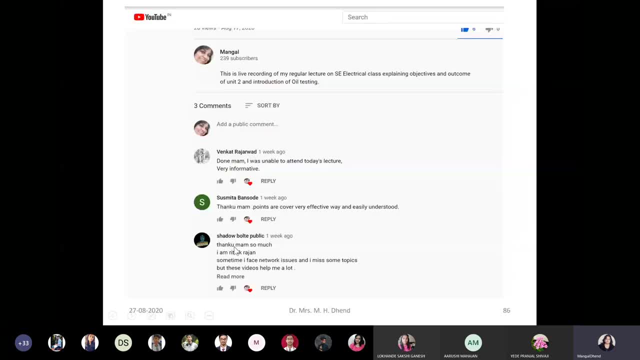 Only two students have given comments. So what Venkatesh is saying done. ma'am, I was unable to attend today's lecture- very informative- And Sushmita is saying: thank you. points are very effective and easily understood. 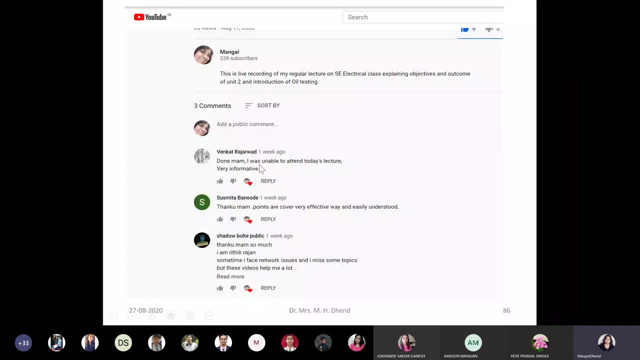 I request all the students, whoever will miss lectures, just go on watching video and go on giving comments so that I will come to know that you have watched videos so that I can consider as makeup lecture. Otherwise, your attendance will be. 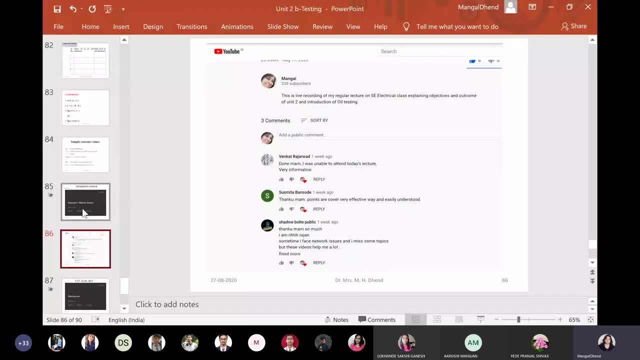 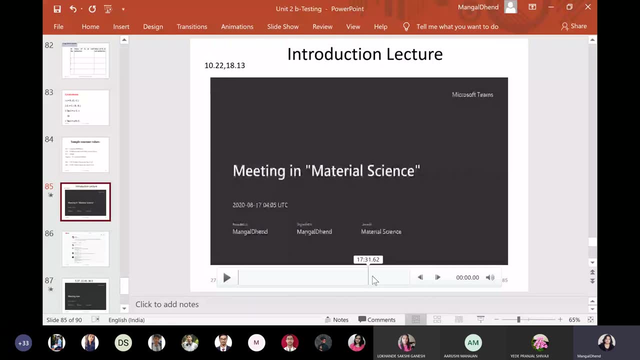 Very weak. just I am reminding you again. So here in this video I just wanted to show you at this. I am just mentioning these points to make me recall which I want to show you. Just see it, Because in my first week lectures, 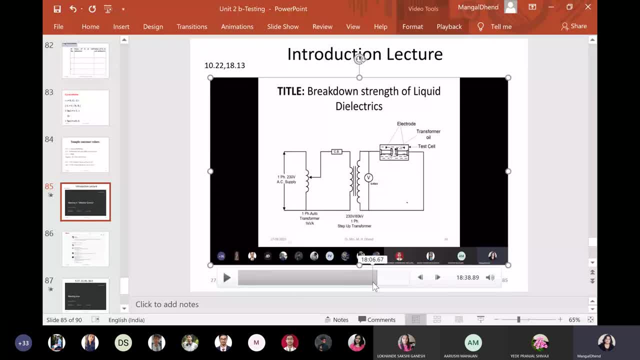 Just it is. So now you want to find out breakdown voltage of liquid Means. what Number of experiments are there on finding breakdown voltage? So you know now insulating material- you know transformer- I Lazy In Insulating material- and when you will place between the two electrodes, to what voltage insulating material will break down, and then you will understand how breakdown has occurred and then note down the voltage. 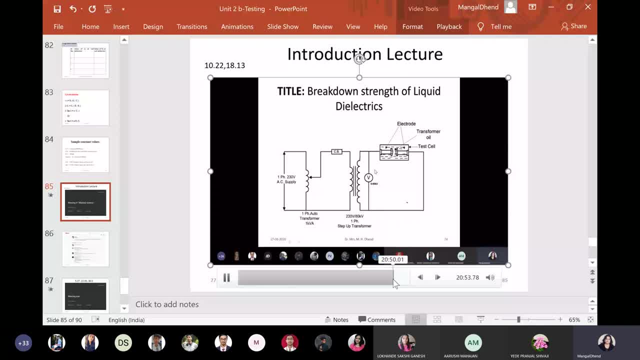 So this whole meter will be memory logging, So memory of that breakdown voltage will be stored on the reading. You just push three experiments except- and what is meant by breakdown? And we will In this diagram, 80 kilo voltage. 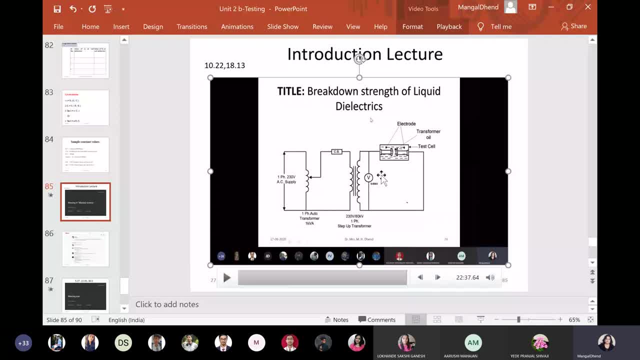 So this is just a general circuit we can use for any testing. But in our lab we will have, we will use oil testing kit. That oil testing kit rating is 60 kilo volt not 80 kilo volt Because separate device. we have to test the oil because we require test cell. 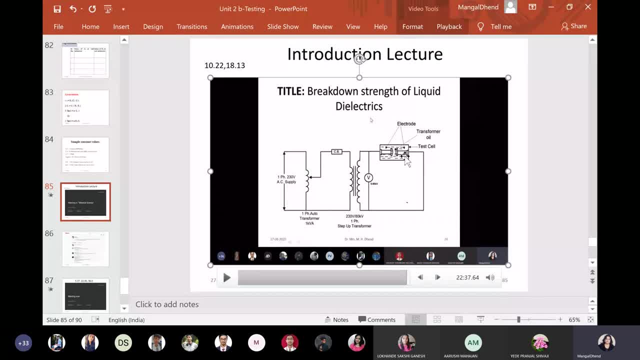 So that kit we will use for testing. Now Simin madam will just take a photo and videos on actual apparatus. I am taking on virtual lab, Okay, So that way also. So we will try to show you what is actual, our test set up and how we can perform that. 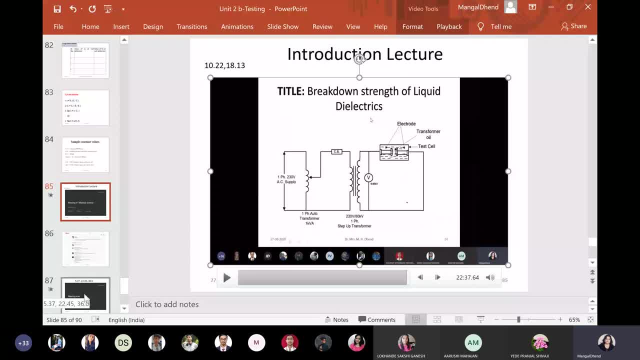 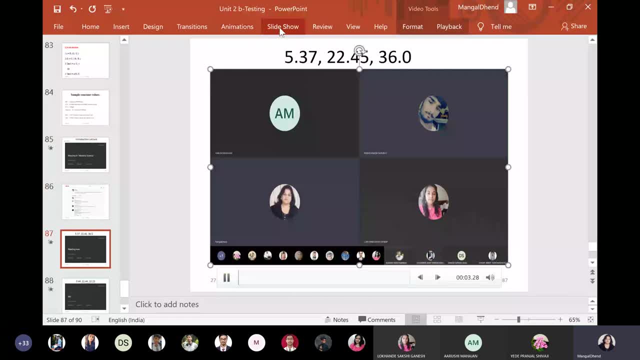 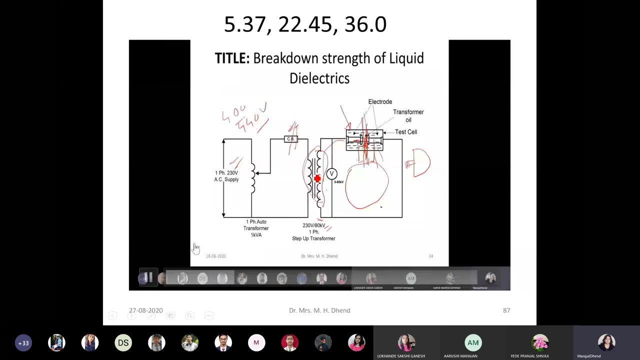 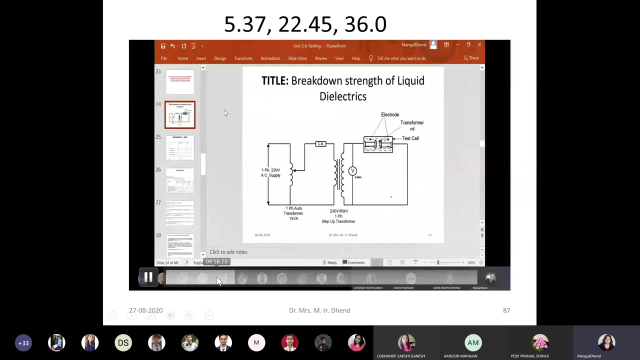 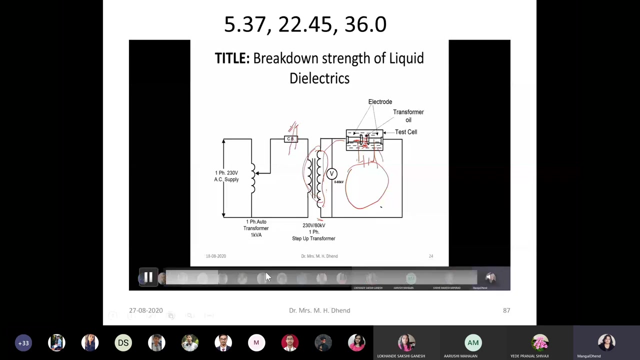 Now let us see this. Our unit, This circuit breaker, is must. So if we want to talk about What will be the equipment's use for finding breakdown strength of transformer oil, First liquid, we should be there, Whatever oil you want to take. 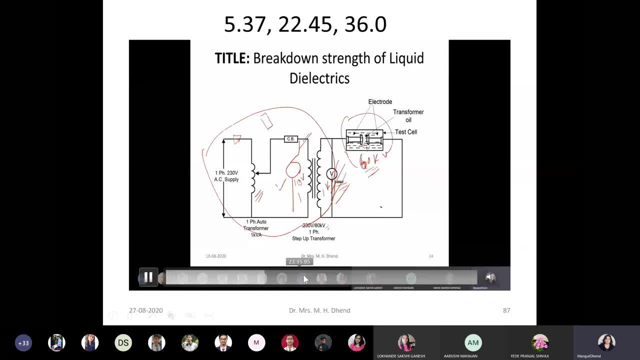 You must tell that actually voltmeter is connected to primary. Now what area exam? Suppose I am between the electrode, Okay, And for a wood having some particular thickness and we are inserting it. This means that electrodes- I already told you it's not cylindrical. 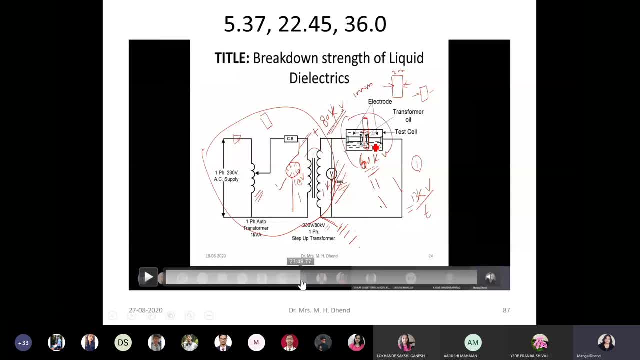 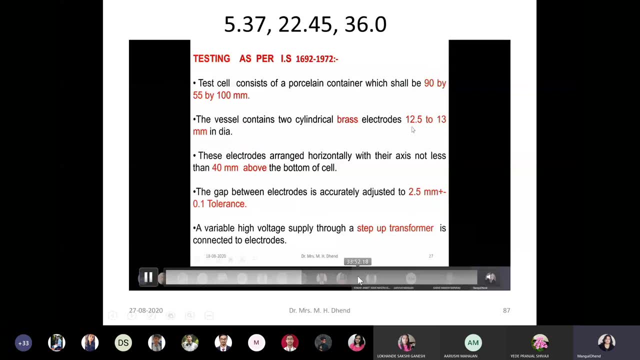 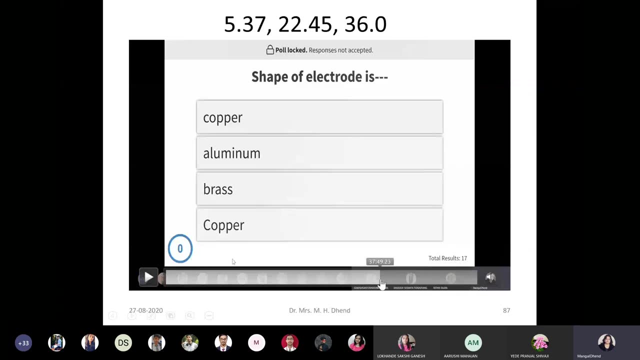 You don't say cylindrical But say mushroom shape, perfect, and dimensions between the diameter of the electrode should be 12.5, 15 finished Now only 17 could respond within the time. Next question: Diameter of elect marks. Now third question: 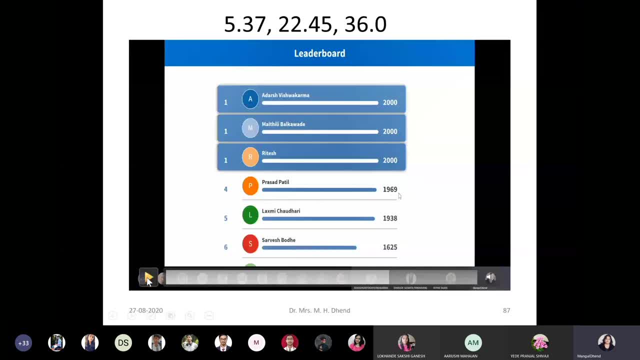 Be ready. So in last competition, leaderboard competition, other show, my Philly, where leading first and then read this cross, or they mean Finally, Retish Was the first. So let us see Now we know who will just. 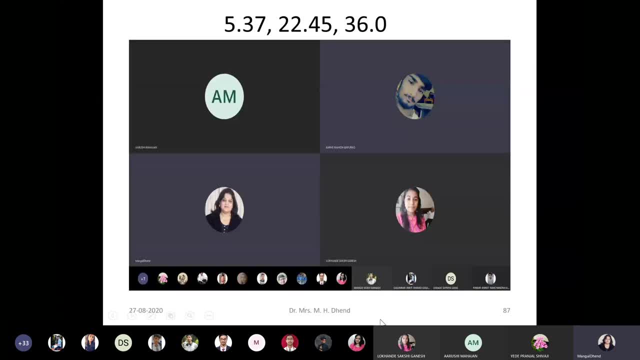 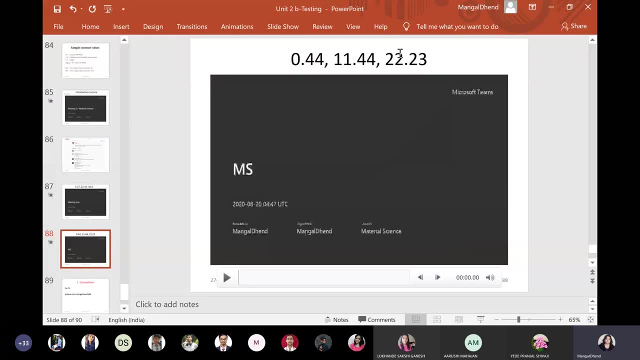 No see, there is a photo. So what happened when I use that to a chill lab and flash? just I made a flash on. I'm getting this problem again and again. I don't know why, But we won't eat that. 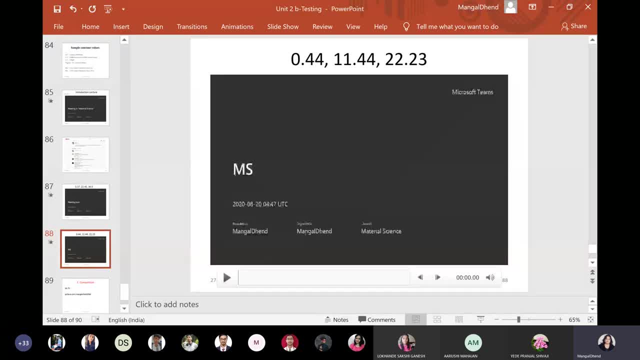 Flash is made off in the setting, Just something is happening to My screen. You tell me what is this problem? Hello, Hello. Yeah, ma'am, You're already. So now what I can do. Can you see my screen? 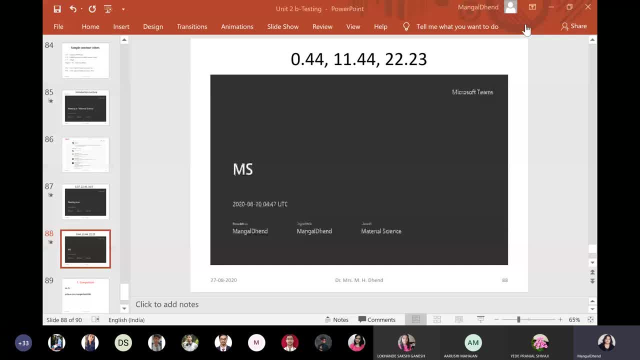 No, ma'am, Yes, ma'am, Oh, ma'am, Yes, ma'am. One minute You can see, but the glare effect is there. I'm getting continue this problem. No, just I'm posting this link in the our WhatsApp group. 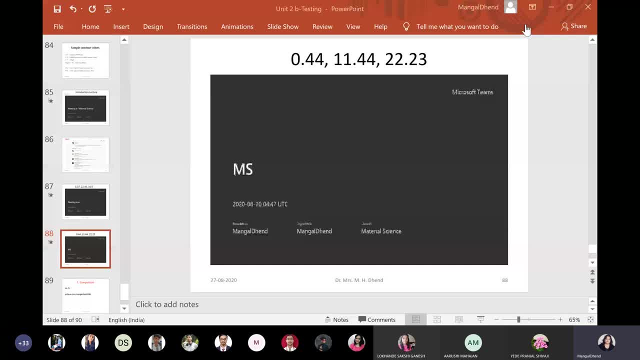 You start giving that test because this flash. Okay, now it's clear. You just call me after our lecture and tell me how I can solve this problem. I'm not taking the same, So do two. No, just so we will just have this quiz. 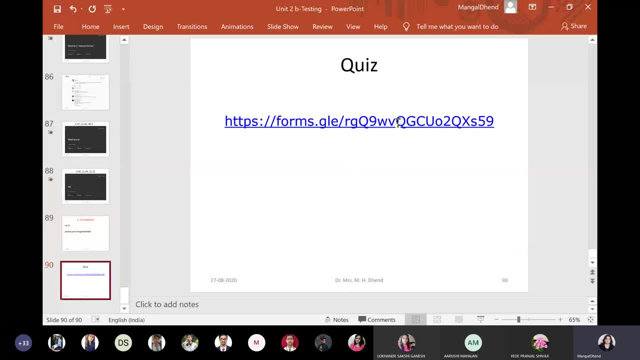 Well, I think first we'll see the competition. So go in for levycom, Dear students. go in for levycom. Use user ID Mangal, then are you at nine For levycom. Be quick, Go in for levycom. 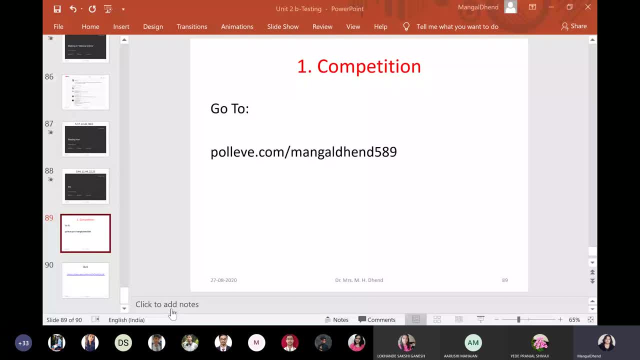 Use password Mangal, then call Mangal. then are you at nine? Okay, Can you see my competition screen? Yes, Are you at nine, Mangal. then user ID: Are you at nine? Yes, Yes, Yes. 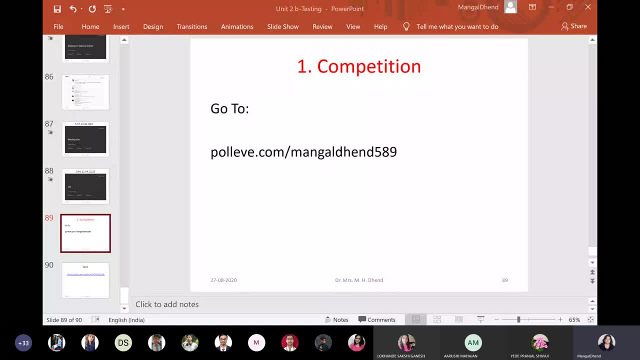 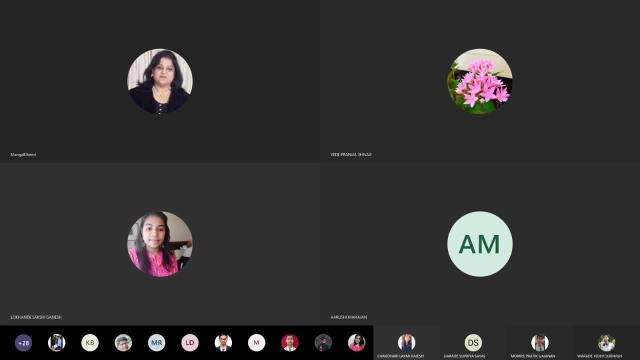 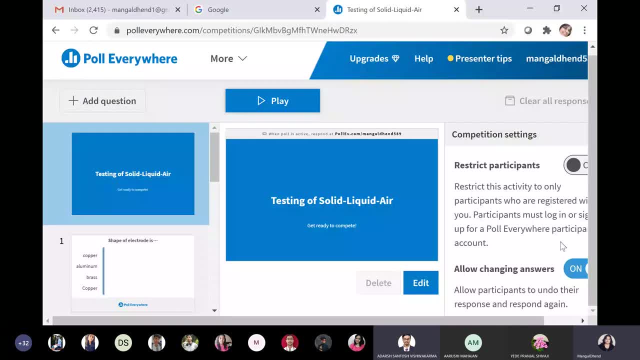 Check all the necessary questions. One question, please. So the important question is this: right now started. So for me. so the the kind of question we are asking That question is is: I know that if you don't know, I can not answer anything without just? 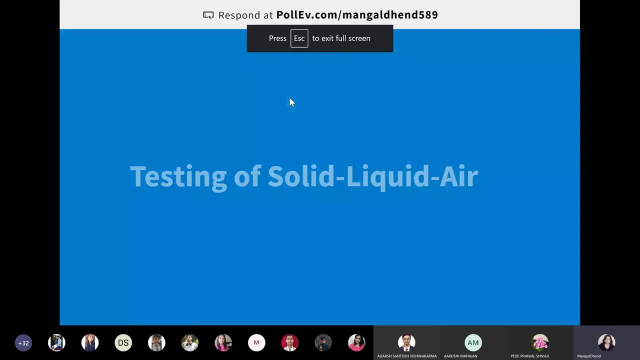 push the button at me, done, Okay. Yes, Can you see my competition screen? Yes, ma'am. Okay, I will start now playing. Be ready. Let us see today who can win competition. Only first top 20 students score will be there. 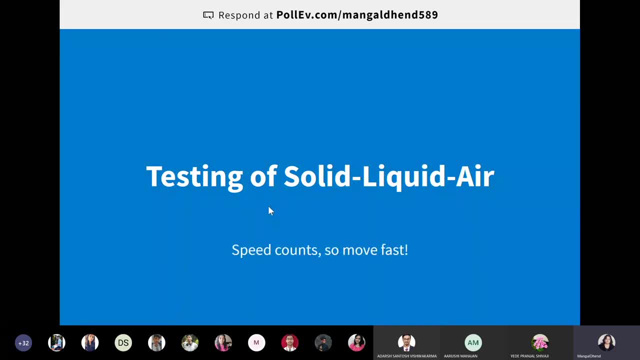 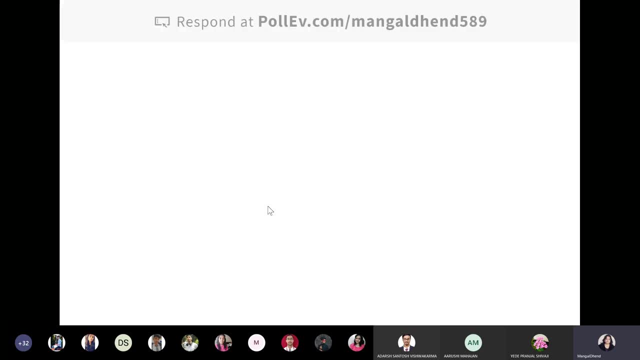 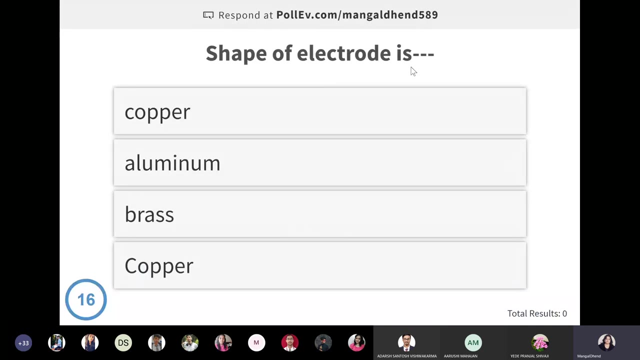 And I will just see who are most 20 active students in our class. So now our competition is on testing of solid liquid air. Now I have started playing. You know time is required. So first question is: shape of electrode is. 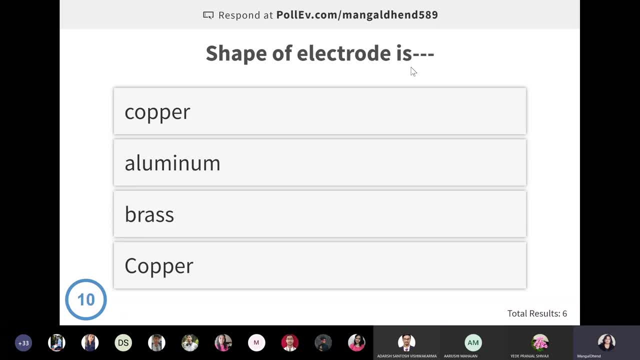 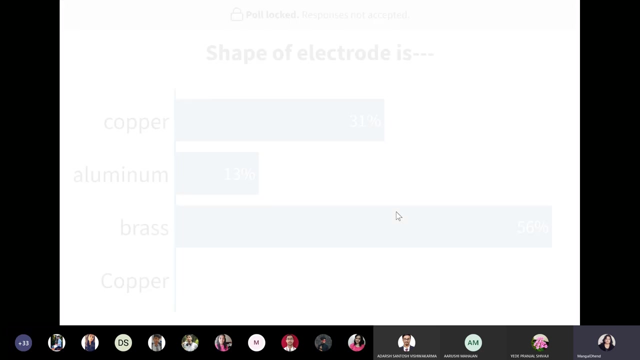 Be quick. Okay, 10 seconds are remaining Only 7 responses. Testing of solid liquid air. Shape of electrode: Okay, only 16 responses. I got Means you are not utilizing full capacity. You might be having range problem, I don't know. 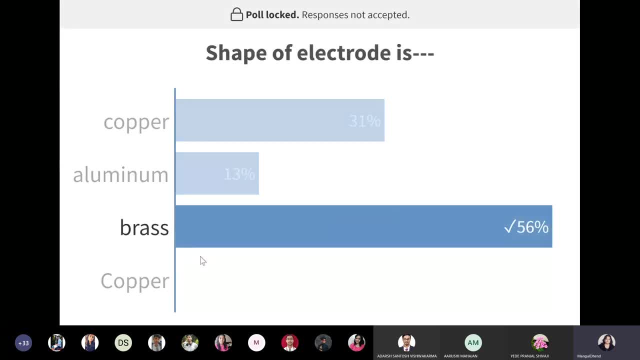 So now just see: brass is the answer, But only 56% of only 16 students could answer correct Means. still, dear students, you need to work very hard. You are not capturing. I have revised it. I show you again the video. 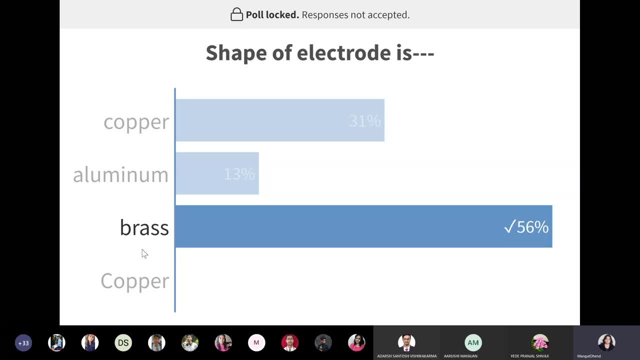 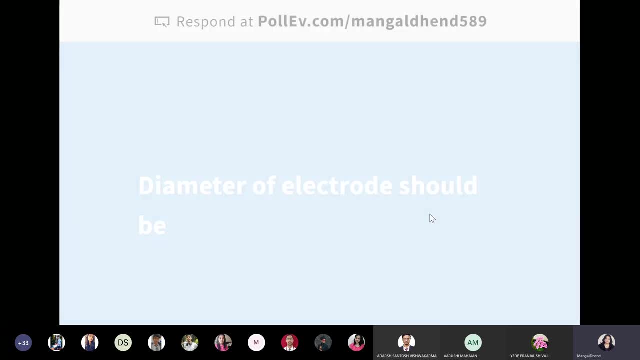 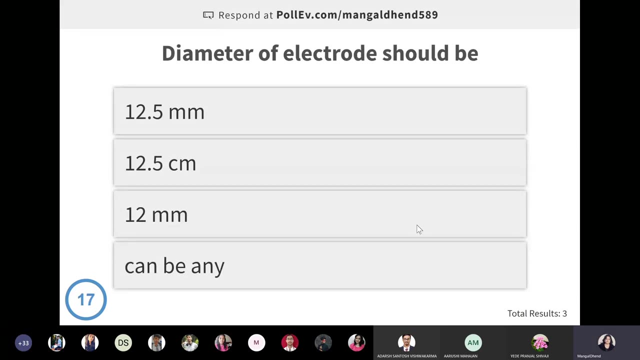 Brass electrode. I just show you that also, But still 31% wrong. And what about remaining students? I don't know. This is about 16 students Now, second question: Diameter of electrode should be At least 20 answers should. 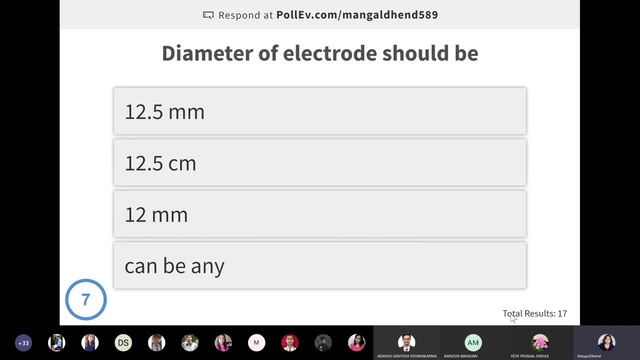 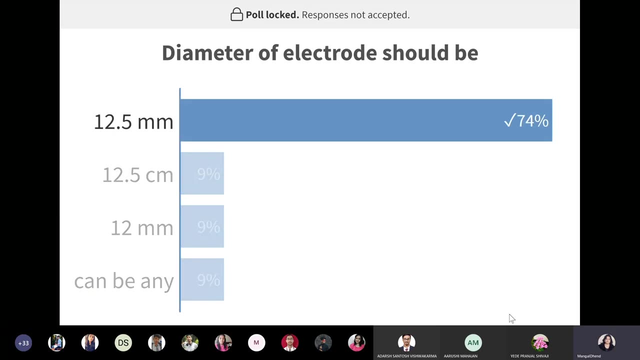 Be there 14, come on. come on 17. good, come on 18,, 19, 20.. Diameter of electrode should be Okay. now answer: 74% students could give correct, But 12 mm. 9% have said and can be any 9%. 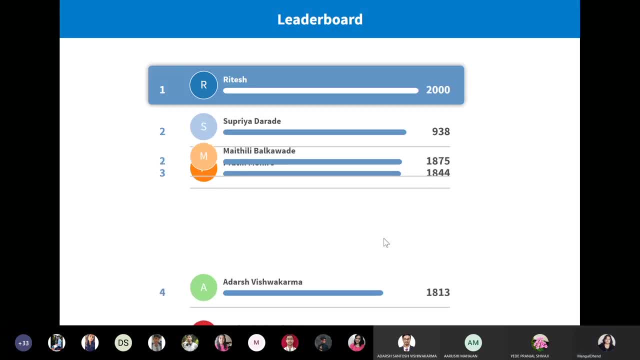 You work hard for Monday's test. You work hard. So again, Ritesh is scoring. very good, Ritesh, Ritesh 2000.. Pratik Very good. Adarsh, What's happened to you? 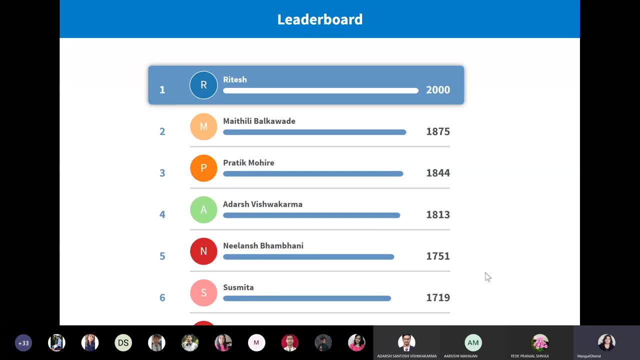 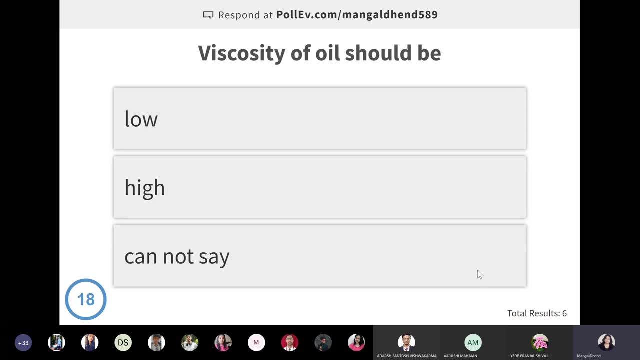 Nilash. Yeah, Good, Sushmita, Good. Okay. Now testing of viscosity of oil should be: Come on fast, fast, fast. Viscosity of oil should be very fast, 20.. Okay, Very fast. 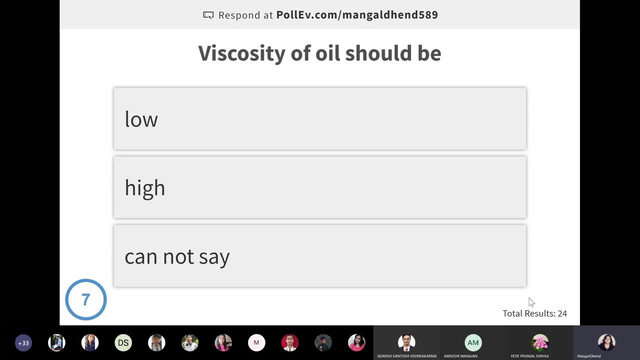 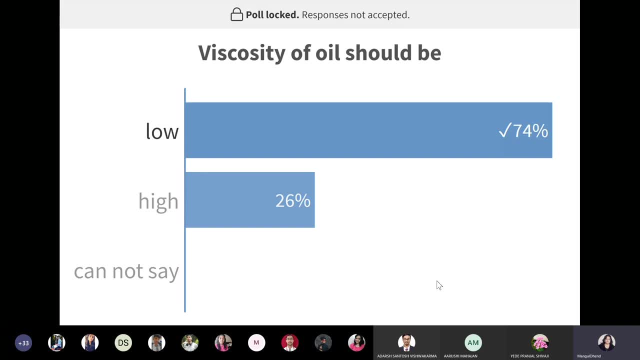 You could give. I think 25 can give 24.. Okay, very good. Now what is about? answer: 74% Viscosity of oil should be low. If it will be high, what will happen? Cooling will not be proper, Temperature of oil will be high and then breakdown will be there. 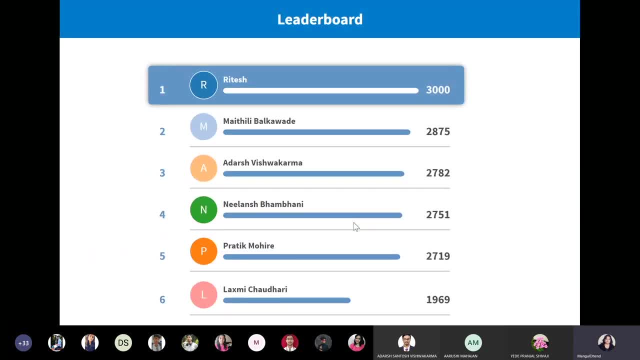 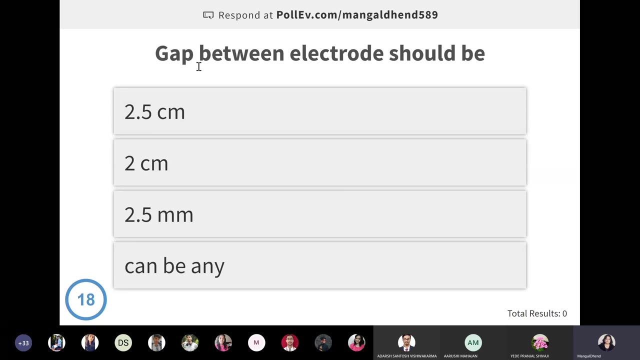 Good, So again Ritesh, Maithili, Adarsh, Nilanj, Pratik, Lakshmi. And what about other remaining students? Only same same names are coming. Okay, gap between electrode should be come on fast, Fast, fast. 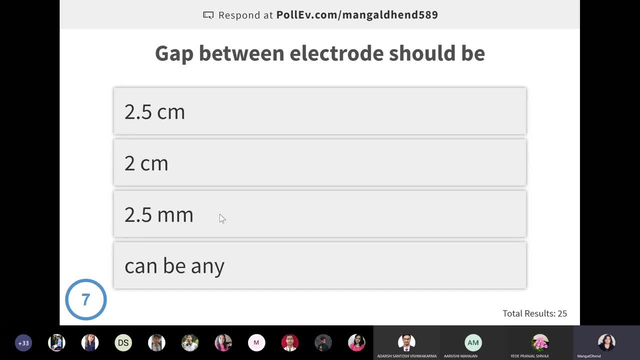 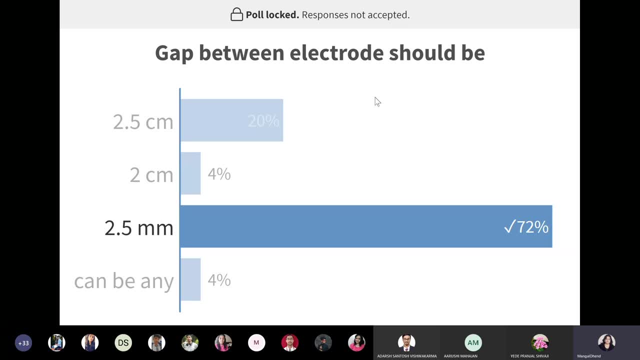 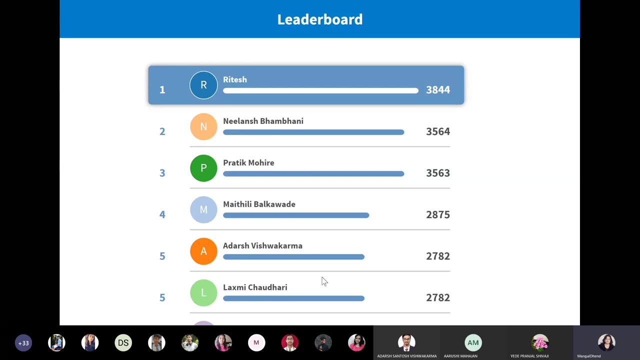 Good. 25 could give Very good. This is the fastest response And 72% only could give correct answer. Gap electrode should be Again: Ritesh Nilanj Good, Nilanj, This you might have given very fast Pratik also very good, Lakshmi good. 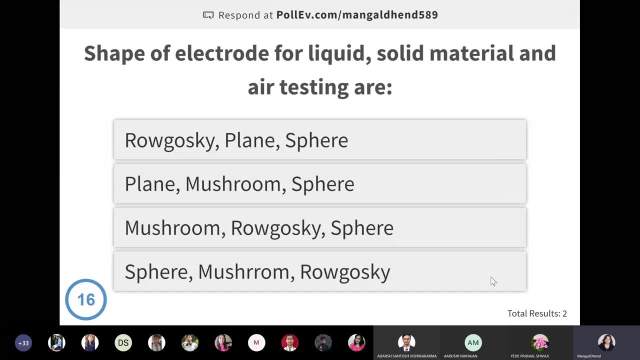 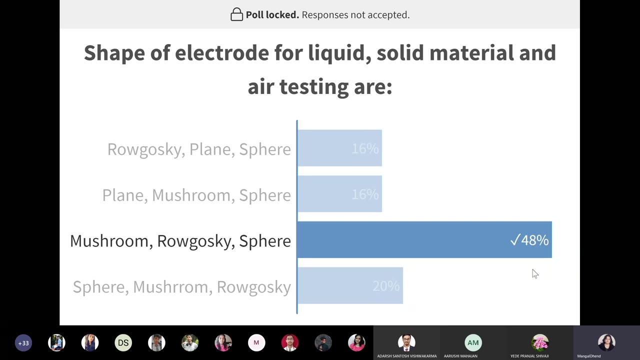 Come on, Shape of electrode for liquid, solid and air testing are, Come on very fast, Only 13,, 14,, 15,, 17, 25.. Very good, So what should be shape? Oh, very poor. 48% only could answer correctly: Shape of liquid is mushroom, Shape of solid is Rogoski And shape of air is sphere, Mind you see. 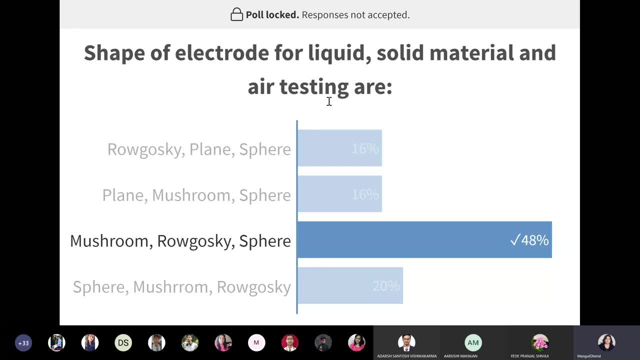 This unique Ir장이 있는, Yes, outside, In the early body. Only one is: salt or saltω. Why is the ball ball? you trippled? why you trippled, you tripped. Okay, what could be? Age, Age: 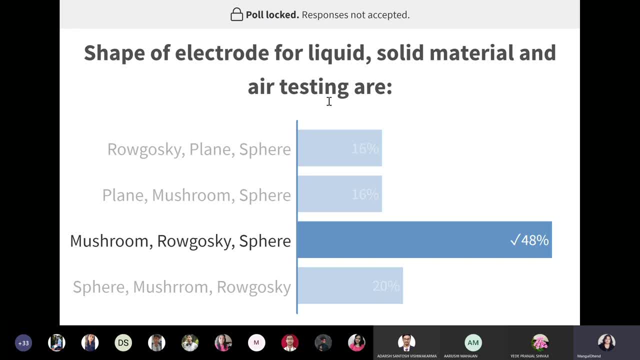 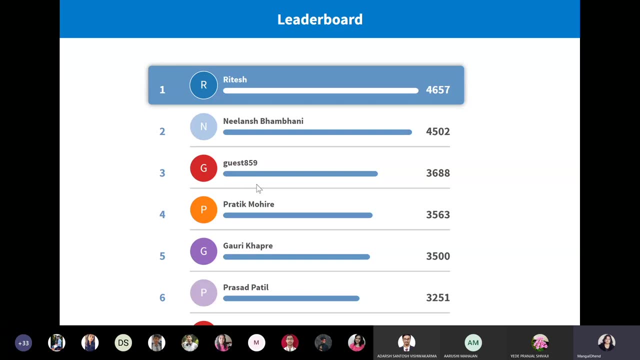 unit is very important. why i am taking revision today again, why i am taking this second test again. competition again monday is there, whether i want to spend time or i want your good performance again. ritesh nilans guest. oh, who is guest? huh, who is guest? can i know our guest? 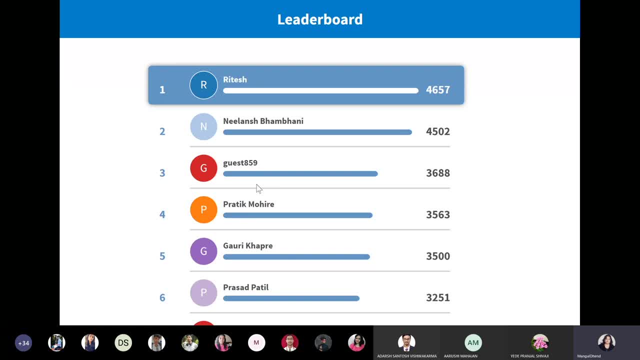 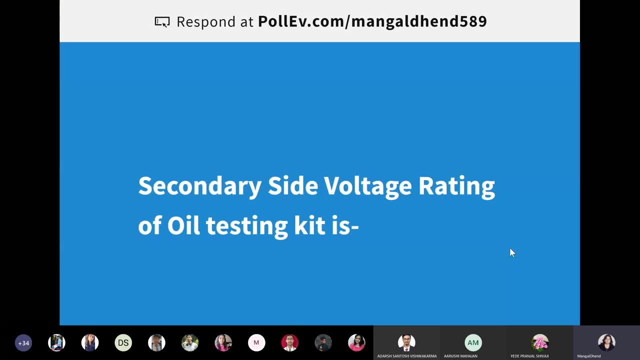 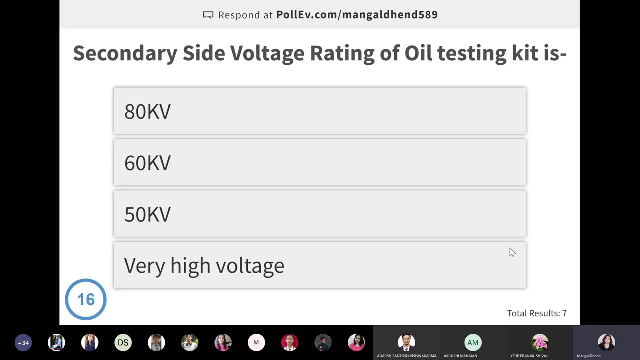 today's guest. oh, samarth, change your login, huh, because you are not guest. okay, now next come on. i have added questions. come on. come on secondary side voltage rating of oil testing kit. just now i told i revised it again purposefully. oh, okay, i revised it. it's 80 kilo old. 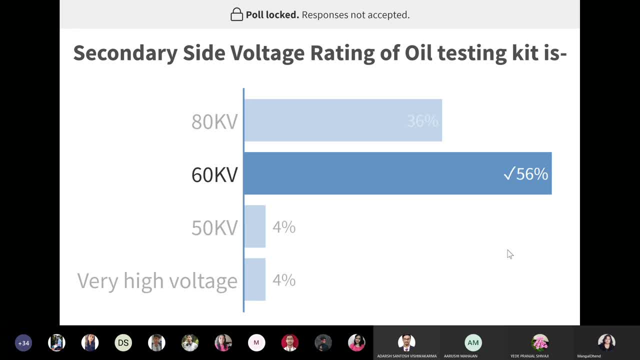 my god, 60 kilo old. oh yes, 60 kilo, 56 percent correct. 80 kilo volt is our college transformer, but oil testing kit is 60 kilo old. i just now told you no means you are not attending lecture attentively. okay, ritesh, congratulations. 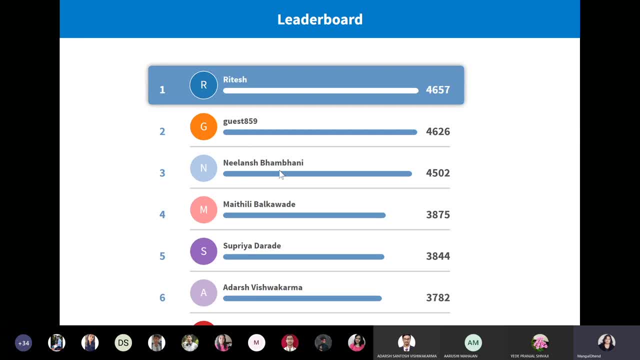 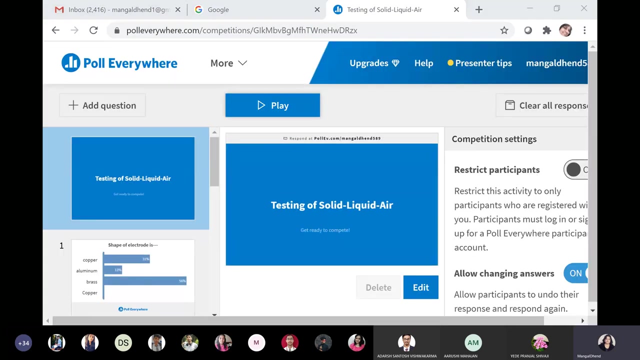 then guest: congratulations nilansh. congratulations maithili, supriya darade. good, very good, supriya, others good six, i can only see, but uh, i will go in mypolyvcom and i will see all 20, okay, okay, just now let us see our ppt. 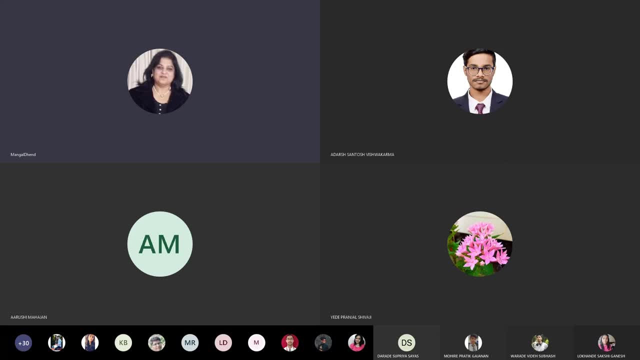 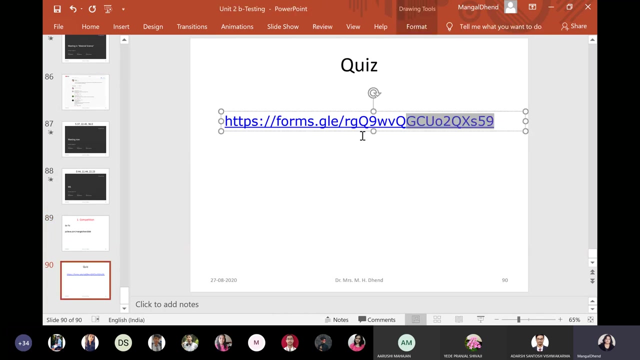 so i have to stop. now again i have to share no ppt, my ppt. okay, competition we are just now. you just uh solve google form google quiz you give. i will post the link in chat box. you take from that chat box and start giving test. be fast. 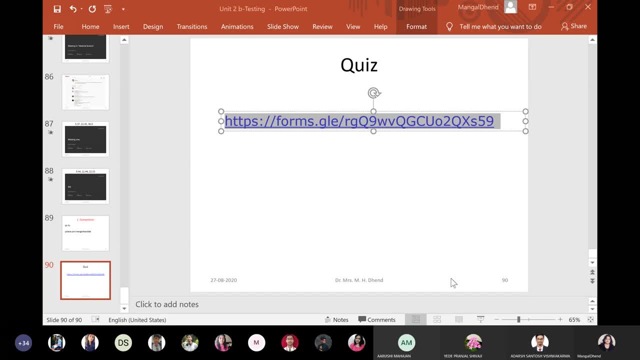 okay, all right, no problem, thank you. so, Students, I have posted a link in the chat box. Student. Hello student. Yes, ma'am, Chat box link is given in. it is also posted in the our WhatsApp group. You start giving quiz. 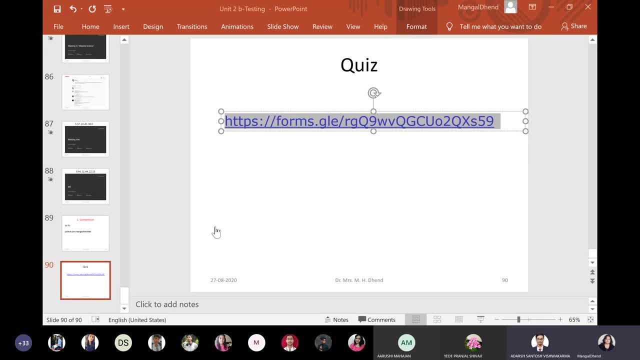 I am giving only 10 minutes. Be fast. Though you seem very busy today, I hope we all get a minute or two to chat. Yes, ma'am, I am in no time. Now you have to keep raising your hand, I am sure. 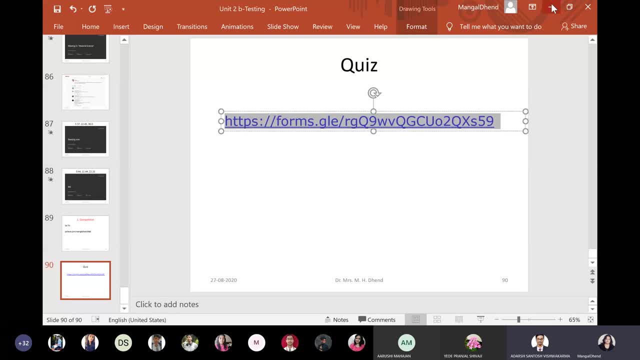 I am really sorry for your bad count. I am sorry for getting you to speak to me. It is all good, No problem, Thank you. I have given you 15 minutes to answer the questions. When you have a chance, let me know. 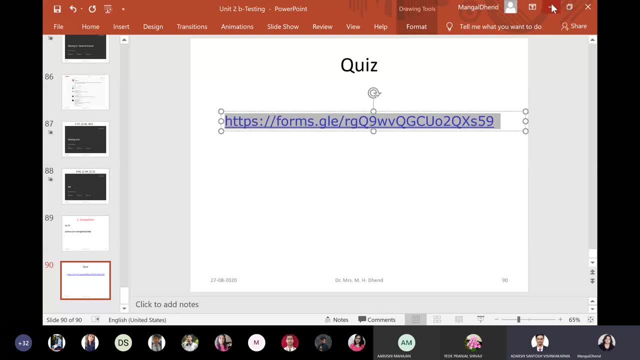 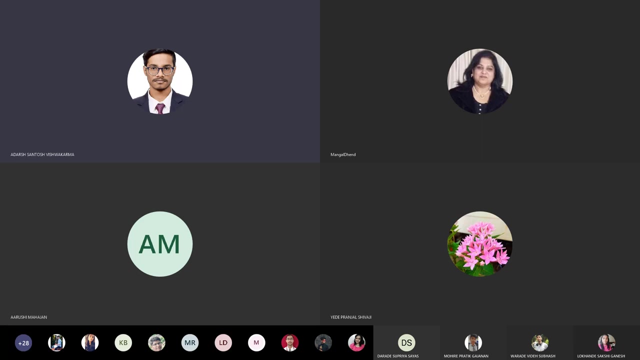 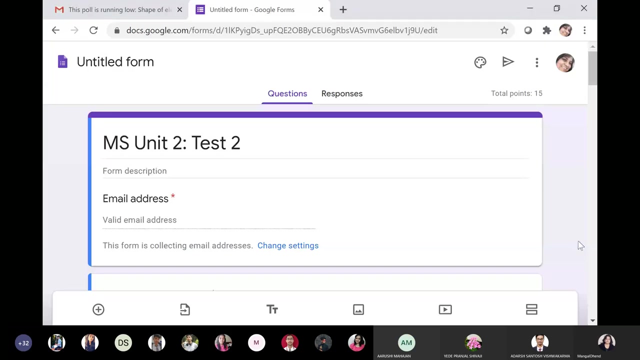 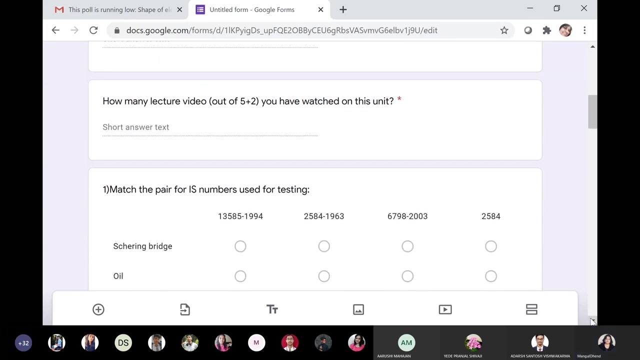 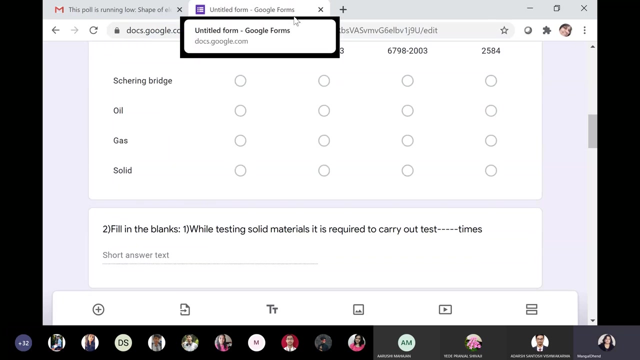 Thank you, Good Thank you. Come on. 15 marks test is there? 10 minutes are there. You just do it. So first write down: match the pair. is there, So you can just match the pair which IS, are you? just? I show you IS number also in revision. 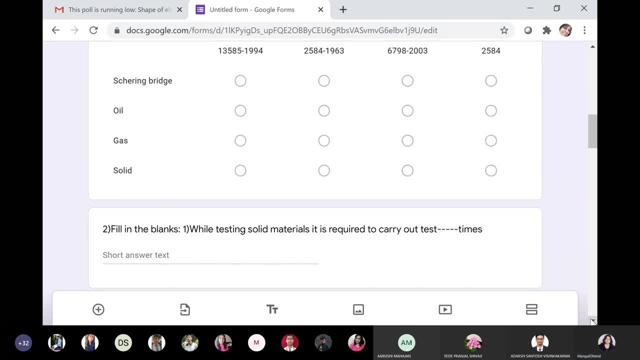 you have to remember IS: just match the pair, Then fill in the blanks. while testing solid material it is required to carry out test dash, dash times. just put number. Don't write down in word because I answer I have given number, numeric value you put. don't write down in word because answer I have given in numeric value. 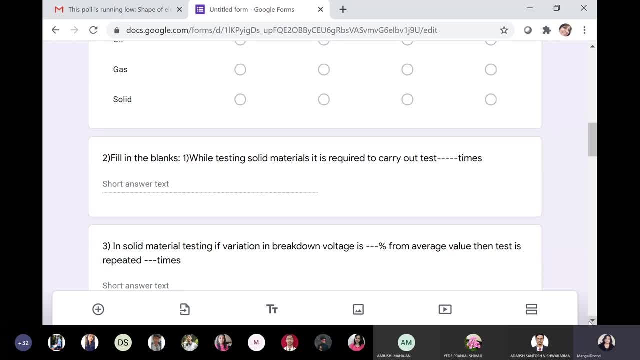 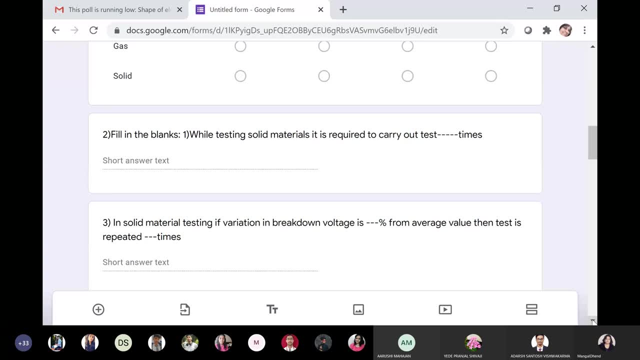 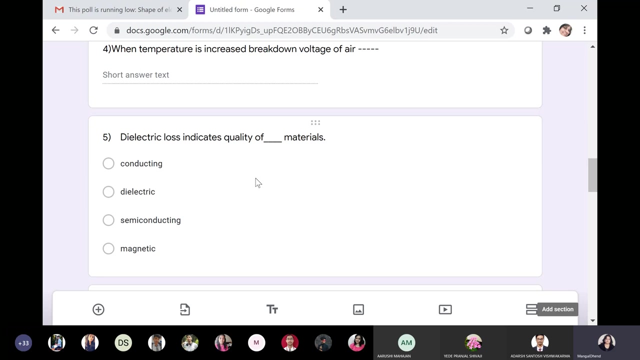 Here also, just write down numeric value for: fill in the blanks, So fill in blanks. And now let's take a look at test. So fill in the blanks, So fill in the blanks. Then dielectric loss indicates quality of material. which material? it indicates conducting dielectric, semiconducting, magnetic. 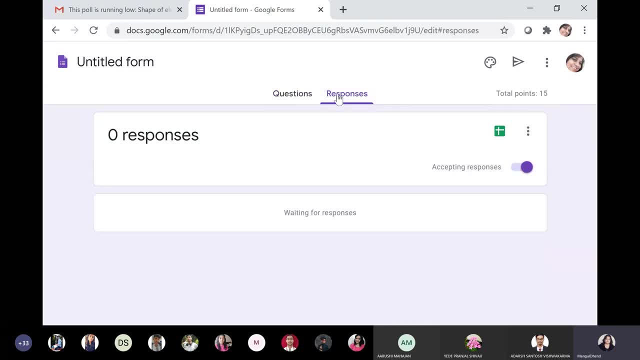 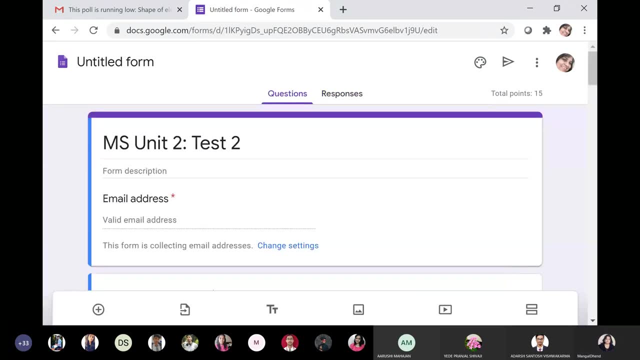 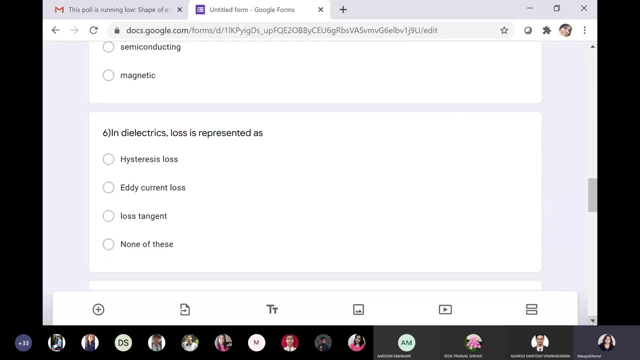 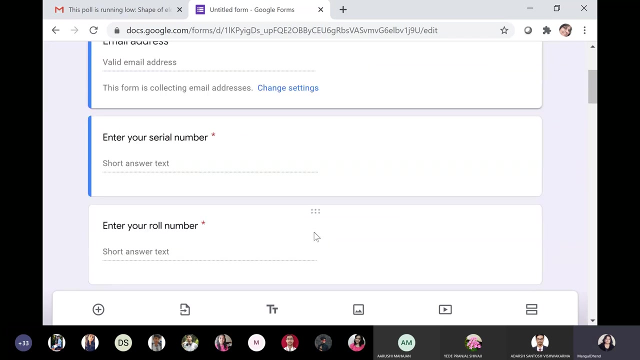 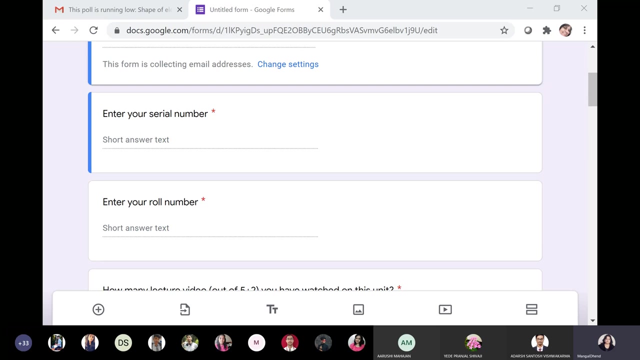 Let me see whether anyone's response is there. No, not yet. You should start giving fast responses. You should start giving fast responses. Eleven questions are there for 15 marks, Because, match the pair, I give four marks. Only 43 students are attending. 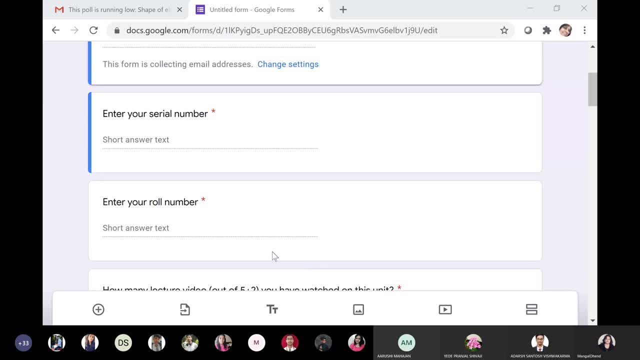 No, I will see the score. I will just post your marks in WhatsApp group. I will close the response after some time And when I will post your mark list, you go through that Again. I will start responses So those who don't have network they can reappear. 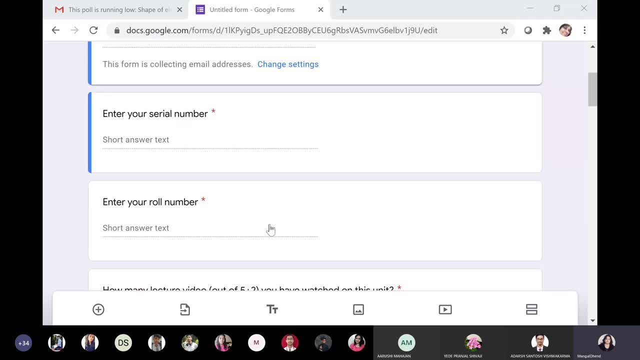 Test And Monday's test marks. I will consider. This is just for practice. I will not consider the today's marks. Monday's test marks I will consider in your term work marks. Okay.